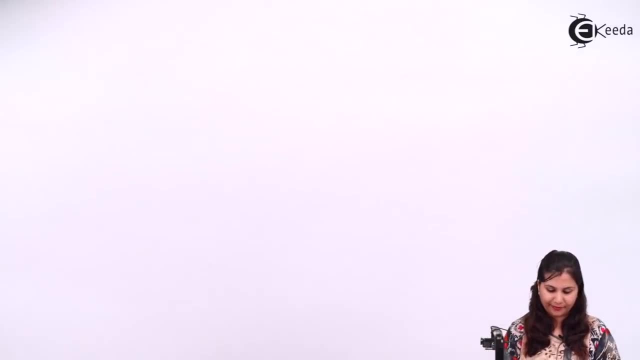 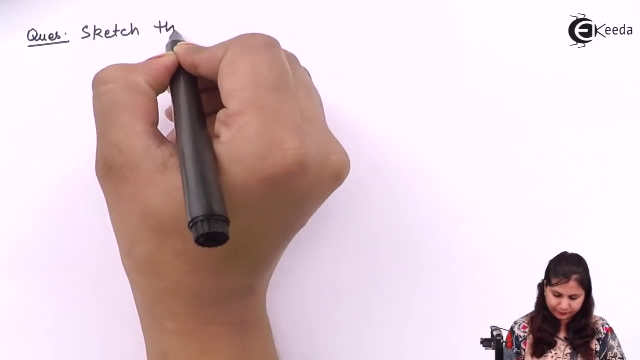 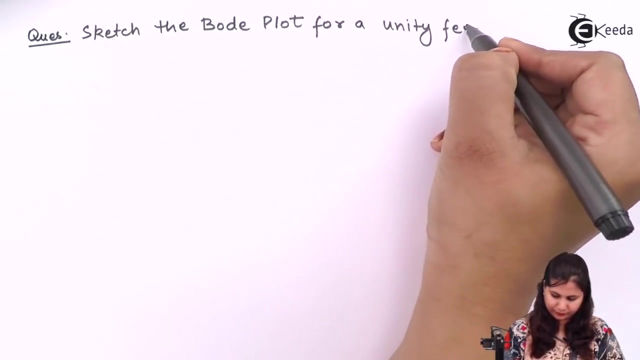 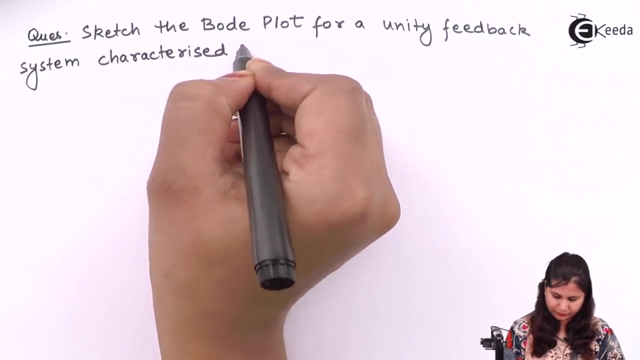 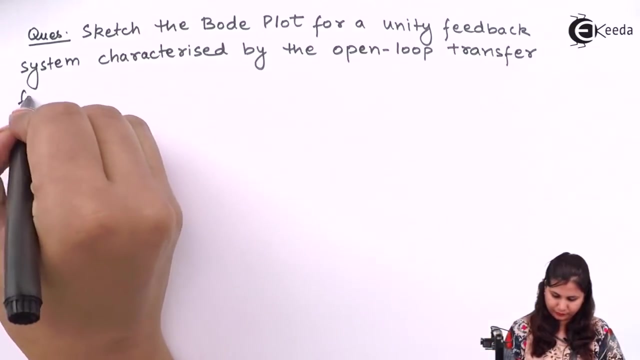 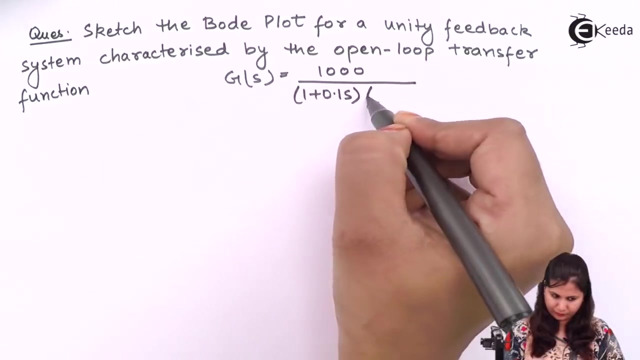 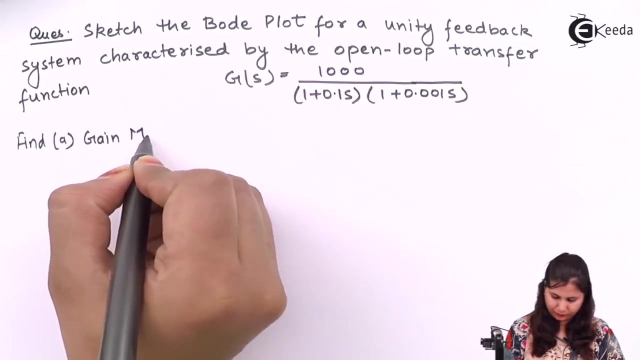 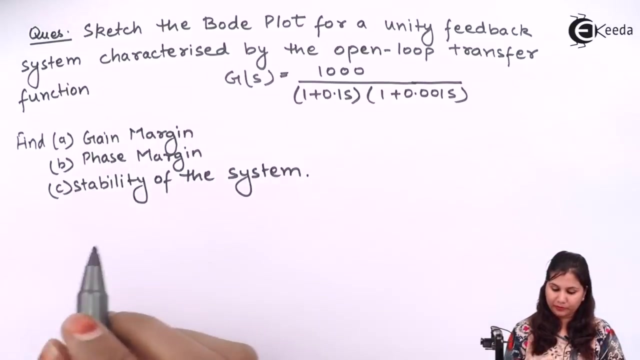 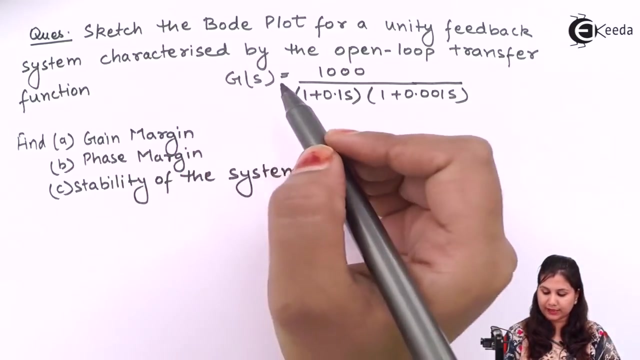 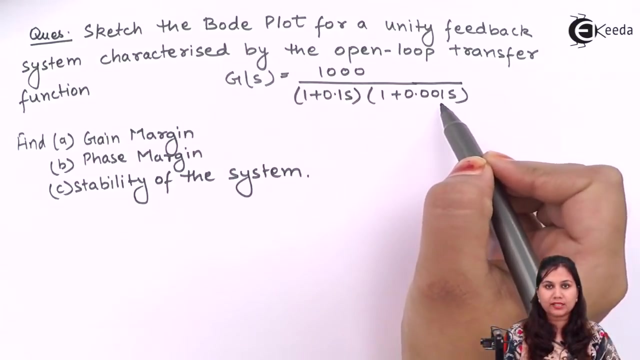 So let's take a problem. So our problem is to sketch the boat plot for a unity feedback system whose open loop transfer function is given to us as gs equals to 1000 upon 1 plus 0.1s, 1 plus 0.001s. We have to find out the. 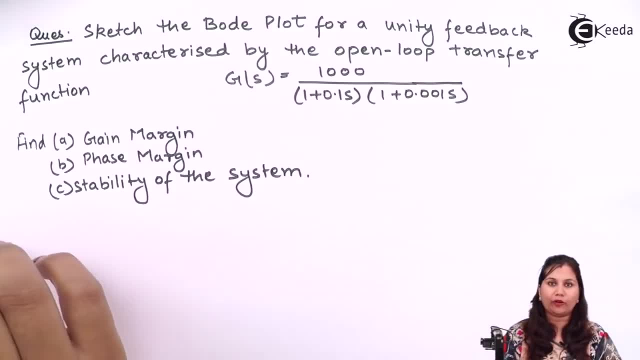 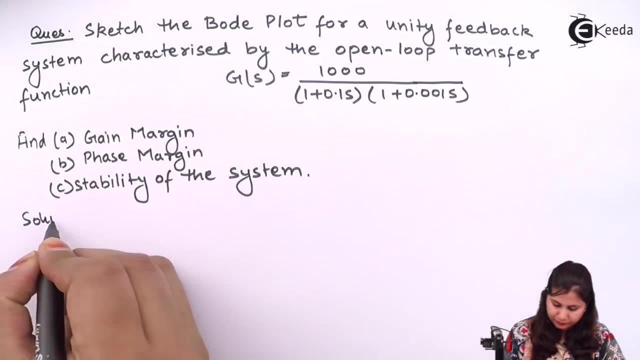 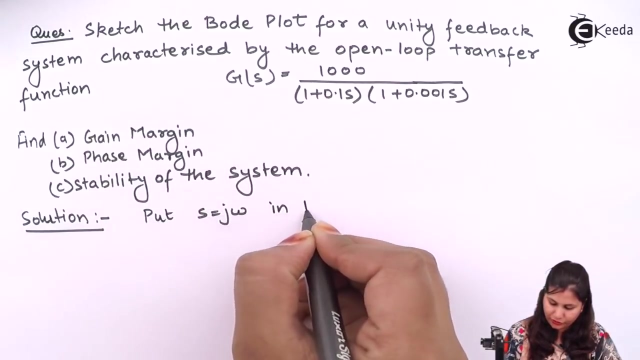 gain margin, phase margin and also the stability of the system. So let's solve this problem. For boat plot. the first step is to put s equals to j omega so that we can obtain the frequency response of the system. So put s equals to j omega in the transfer function. 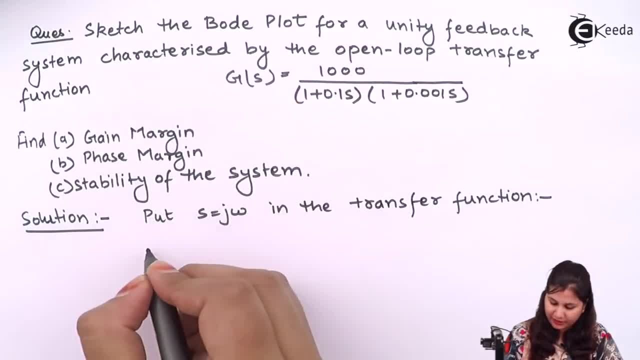 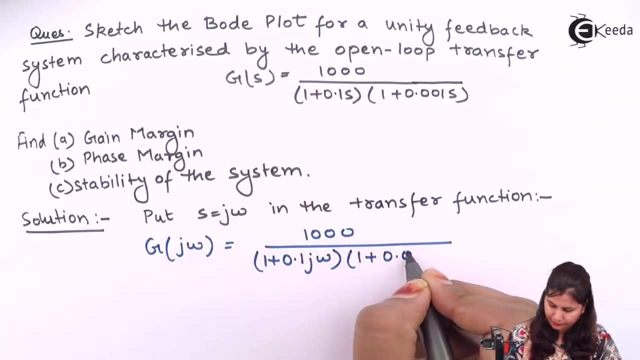 We will get the frequency response, that is, g j omega. as sorry, here we are going to have j omega also. So this is our frequency response of the system, that is, 1000 upon 1 plus 0.1 j omega and 1 plus 0.001 j omega. Now step number 2 will be to find 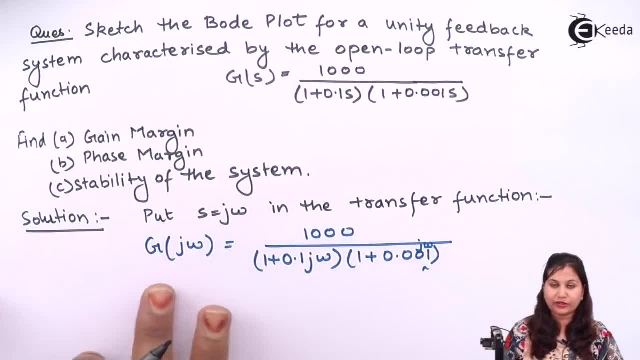 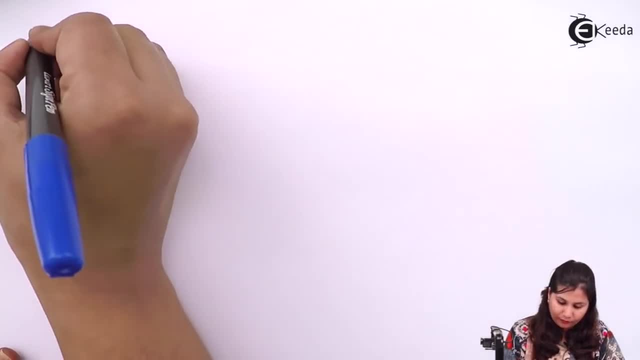 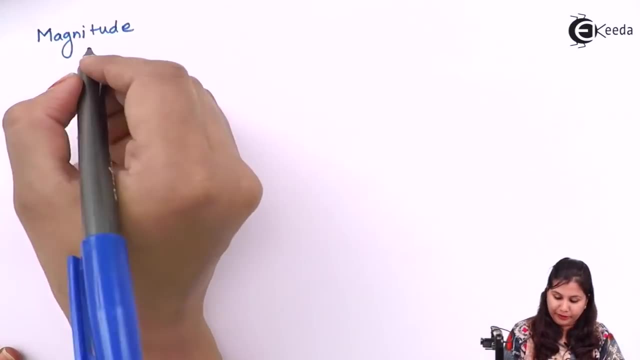 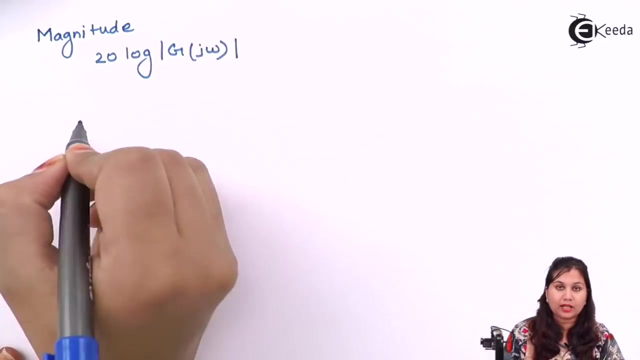 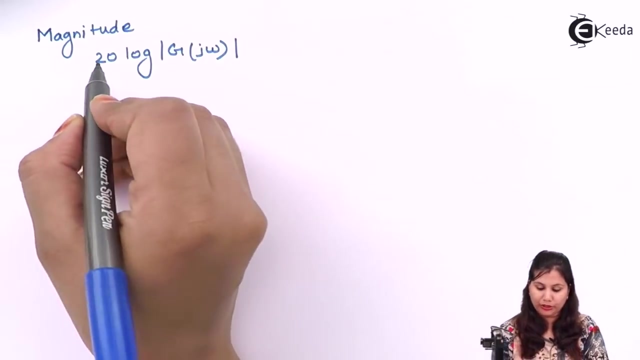 out the magnitude and the phase angle of this g j omega. So our next step will be to find out the magnitude. Magnitude will be 20.. Magnitude will be 20.. Log g j omega. This is the magnitude of g j omega, and here we are taking the logarithm of the magnitude. 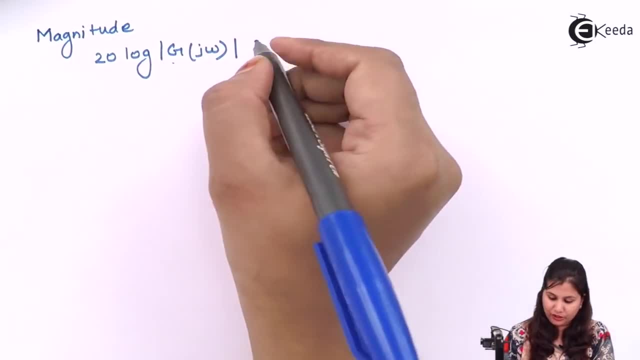 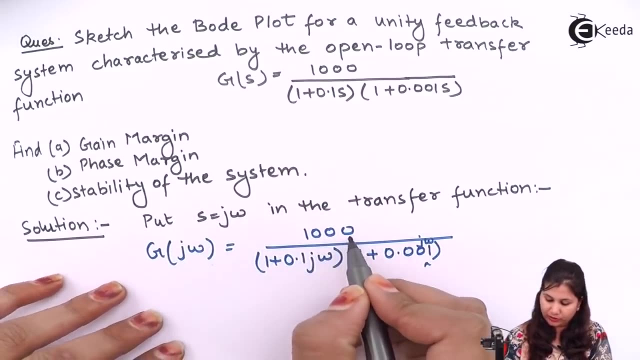 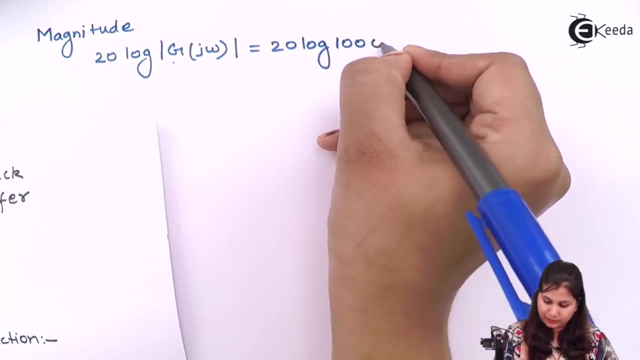 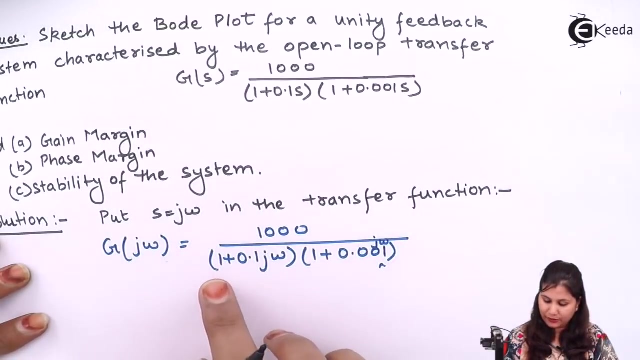 So it will be 20 log the magnitude of g, j, omega. So it will be here in the transfer function we are having the constant term 1000., So its magnitude will be 20 log 1000.. Now for denominator. we are going to have the minus sign, So minus 20 log. This is a complex. 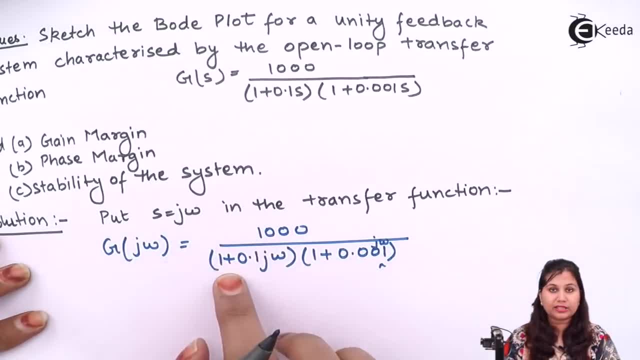 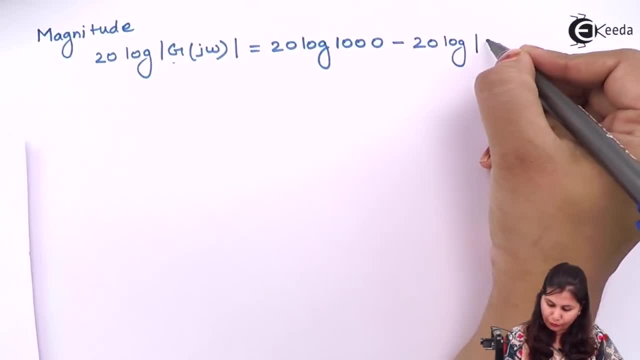 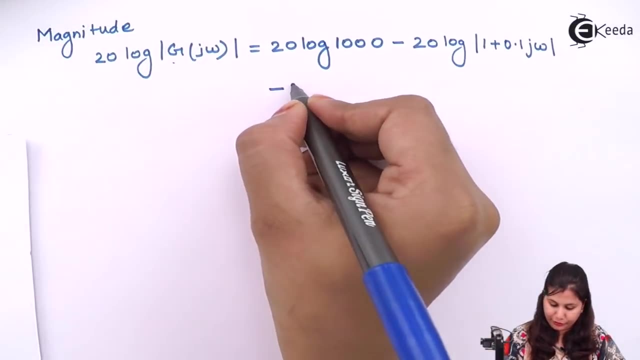 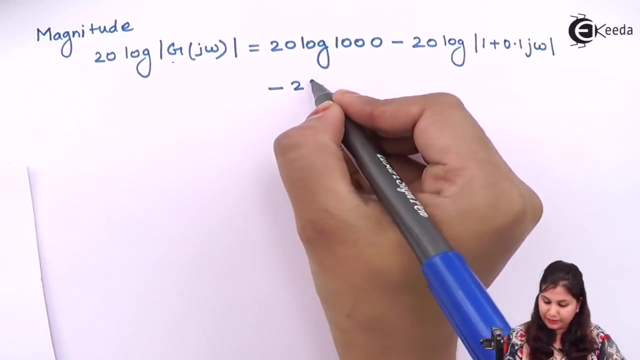 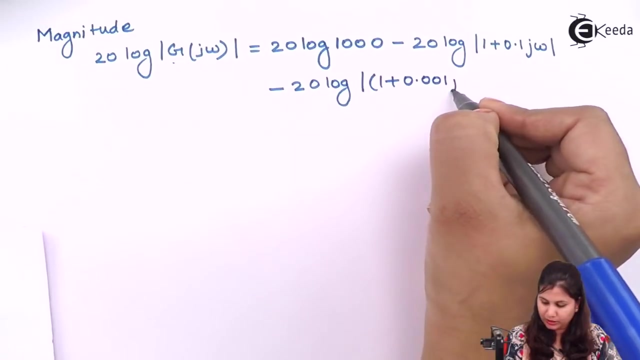 number, having both real and the imaginary parts. So we will take the magnitude of this complex number minus 20 log. magnitude of 1 plus 0.1 j omega. Similarly, magnitude of this third factor, 1 plus 0.001 j omega, will be minus 20 log. 1 plus 0.001 j omega magnitude. 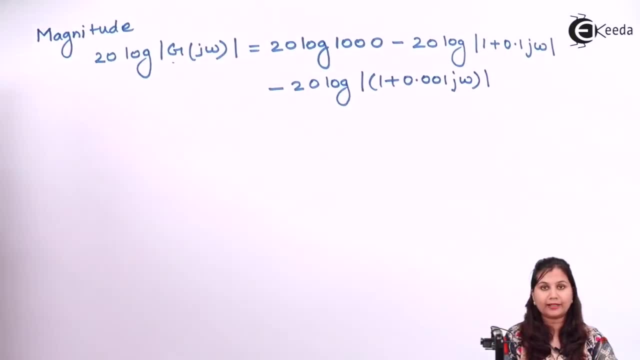 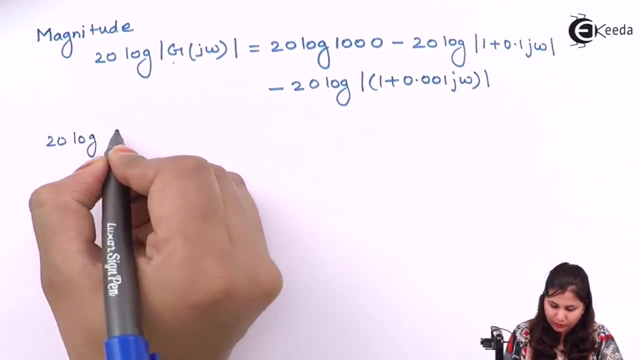 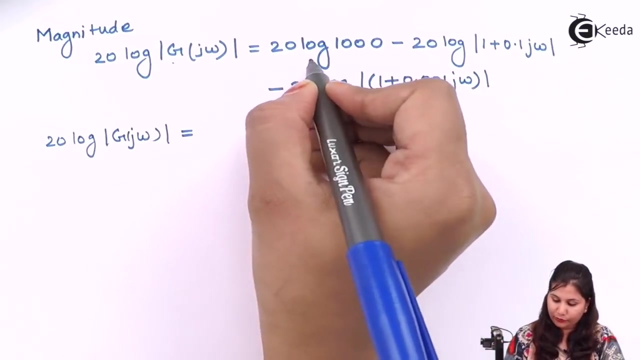 So we have taken the magnitude and then we have taken the logarithm of the magnitude. Okay, Now let's solve it further. We have 20 log g j omega. So we are going to have the g j omega, 20 log 1000. its value will be: if we calculate it, it will be 60, because it will become 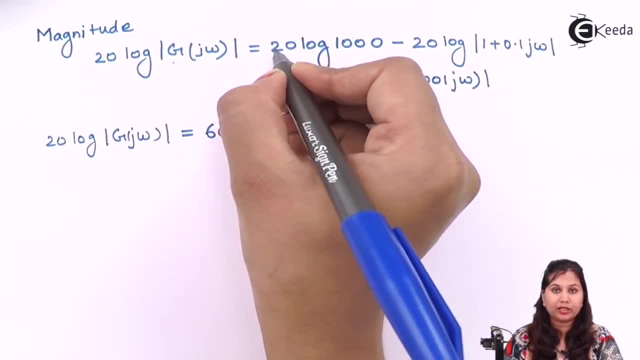 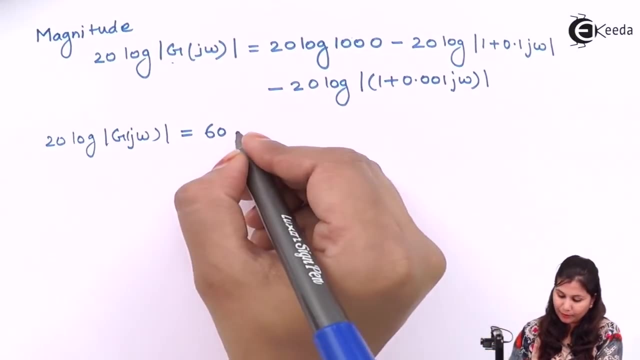 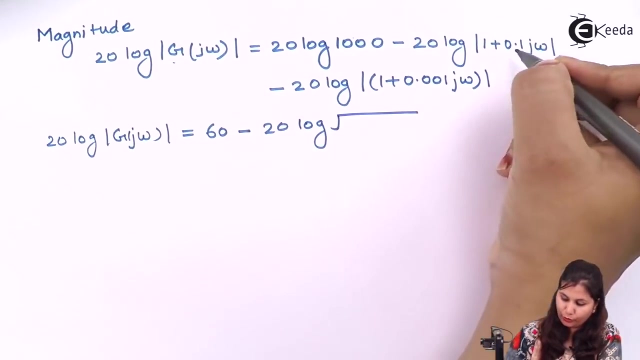 20 log 10 raised to the power 3, so 3 will come in front, so it will become 3 into 20, that is 60 and log 10 is 1 minus 20 log. this is the complex number, so its magnitude will be under root of. 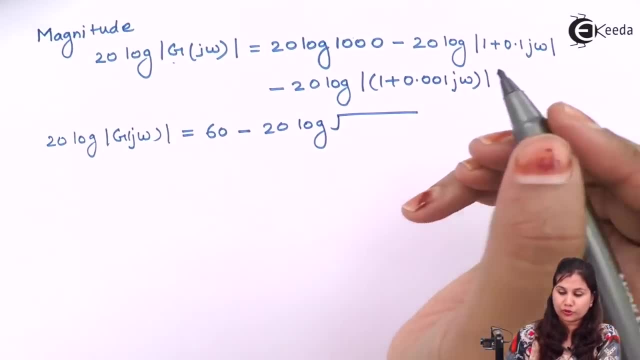 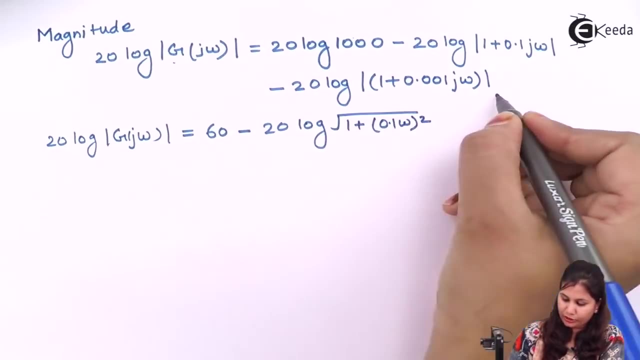 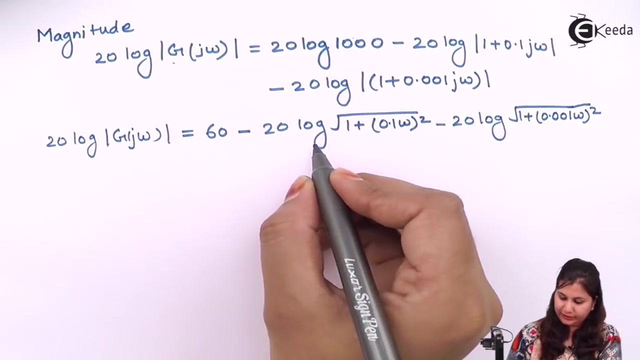 1 square plus 0.1 j omega square, omega square, so it will be 1 plus 0.1 omega square. for this we will have minus 20 log under root of 1 plus 0.001 omega square, so we have calculated the. 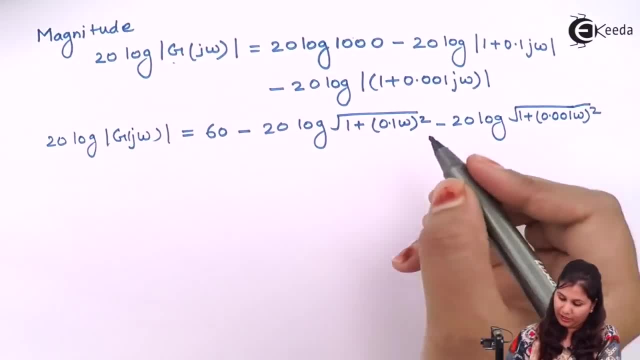 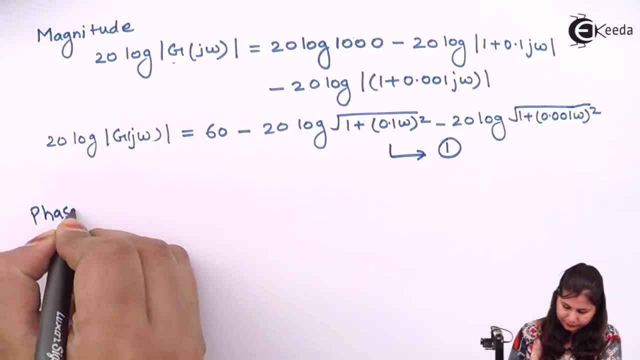 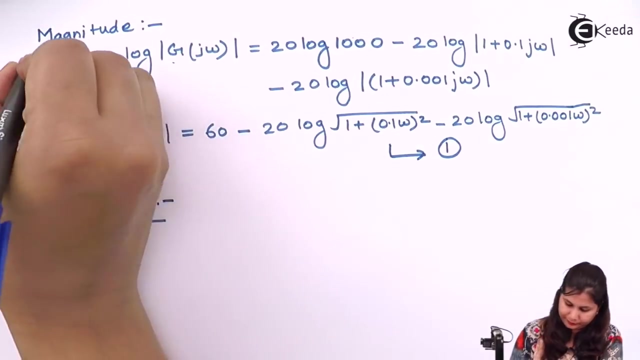 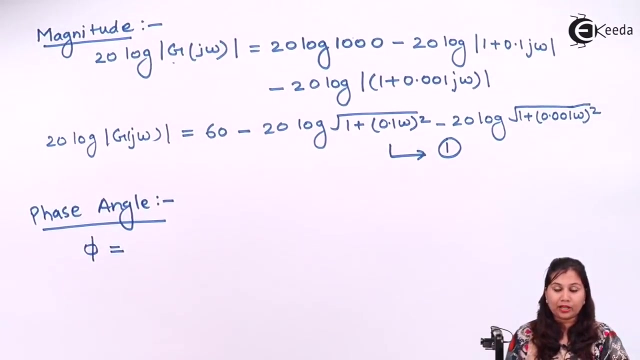 logarithm of the magnitude of j, j, omega. and this is our first equation. now, phase angle: phase angle will be given by, represented by phi, and it will be the tan inverse of the constant term. constant term is 1000, so it will be tan inverse of, because 1000 is the real part there. 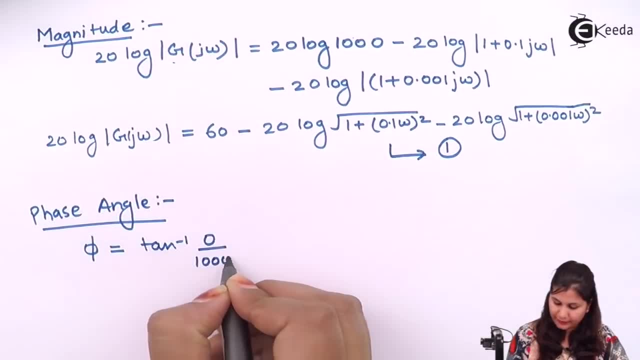 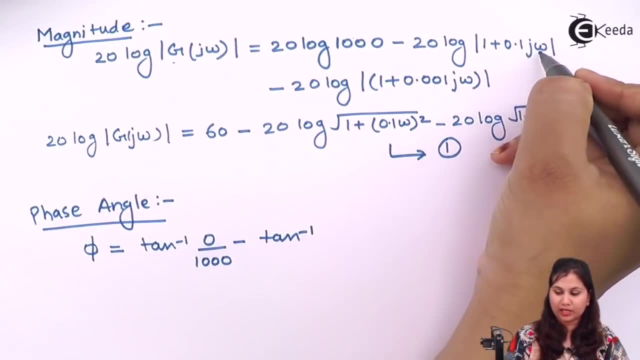 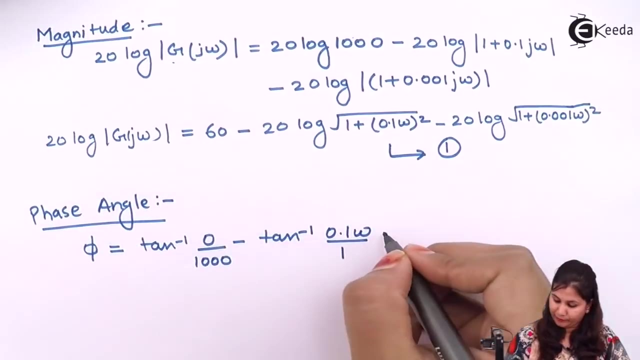 so tan inverse of 0 upon 1000, then minus tan inverse of. here we are having the imaginary part as 0.1 omega and the real part is 1. so tan inverse of imaginary part upon the real part, minus tan inverse of imaginary part, is 0.001 omega and real part is 1. 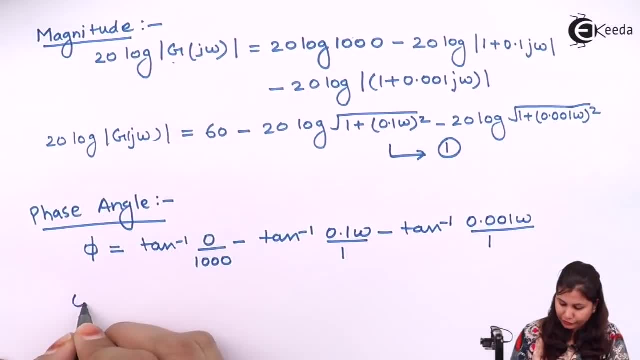 so this is the phase angle. let solve it further. we have phi. equals to this will be tan inverse of 0, so it will take 0 degrees, then tan inverse of 0.01 omega. so about tele道, swoosh point, zEEd og one. 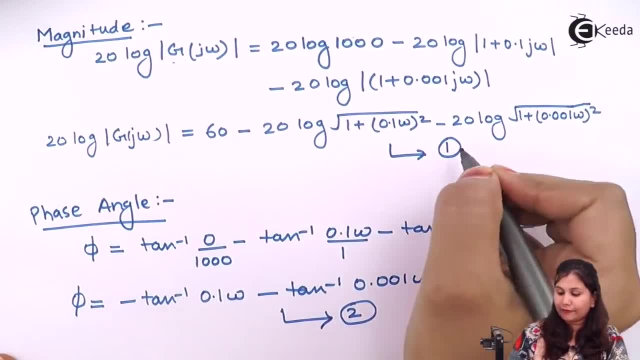 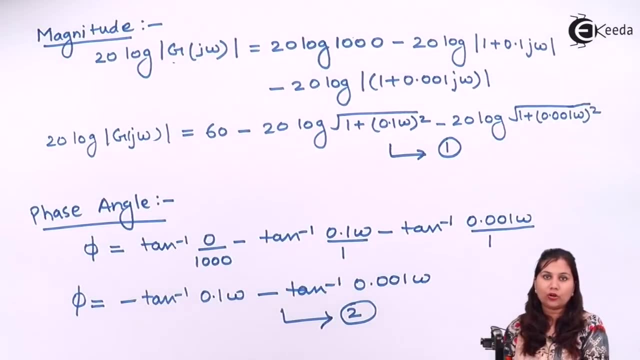 mark this equation as so. we have two equations: one is for the resolution and the Newton quantity from theкимographic t magnitude s, 0.001. phenomenal nog is for the phase angle of the transfer function Gjω. Now we will use this magnitude equation. 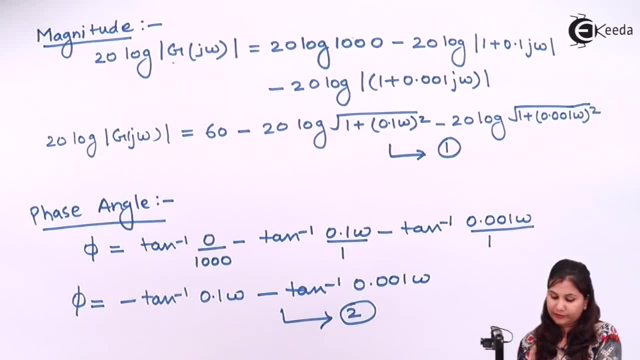 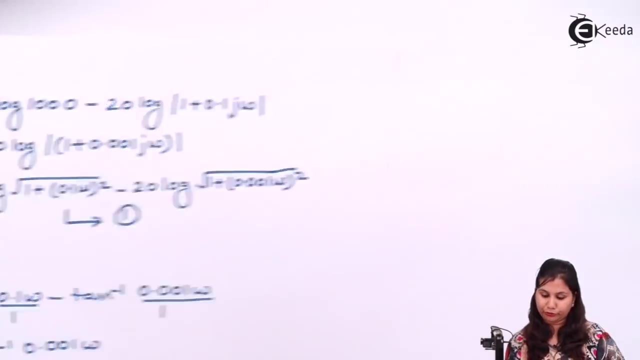 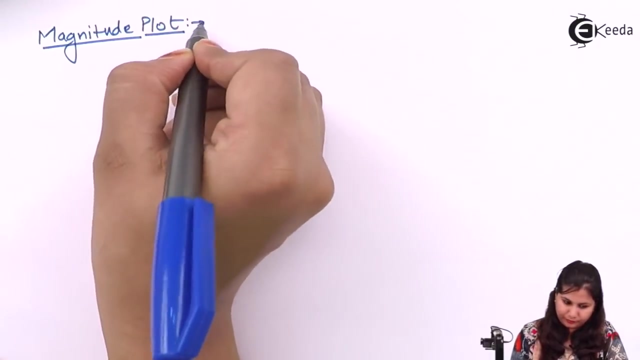 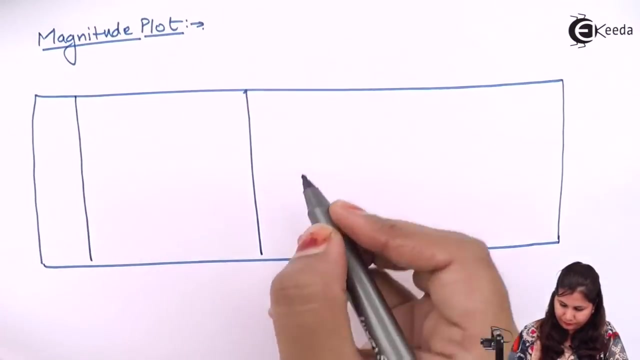 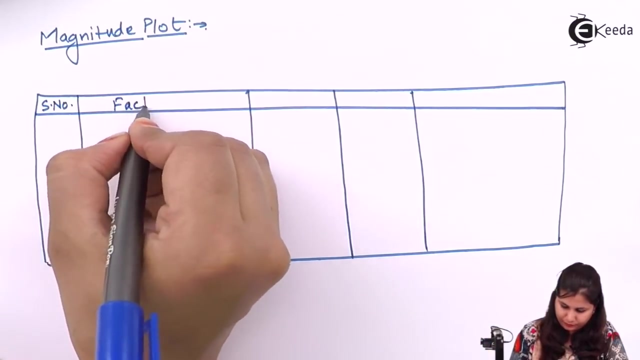 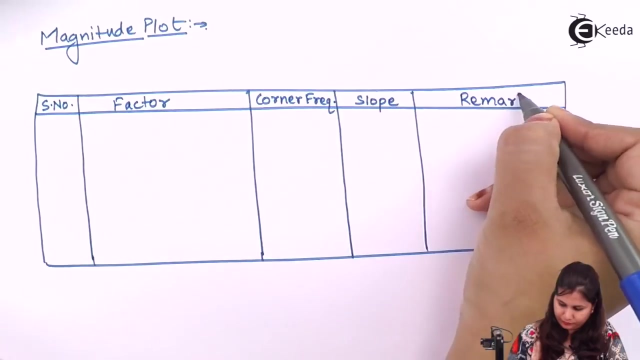 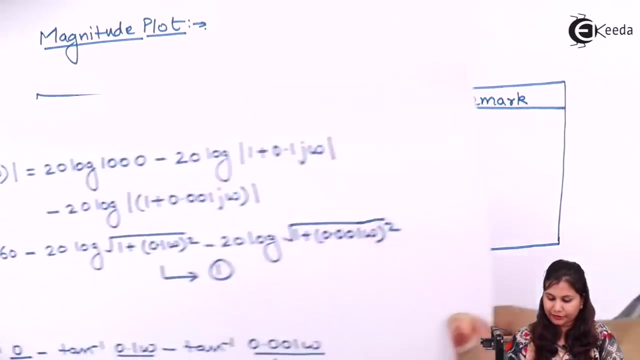 to form a table so that we can- this table is going to help us in drawing the boat plot and this phase angle equation- we are going to form another table for the phase plot. So first form the table for the magnitude plot. So here we will use the magnitude equation. our magnitude equation is this: 60-20 log. 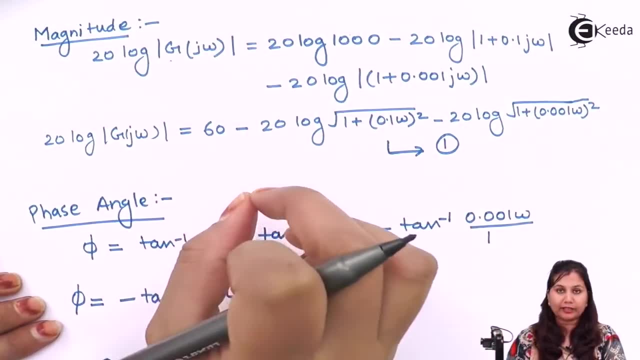 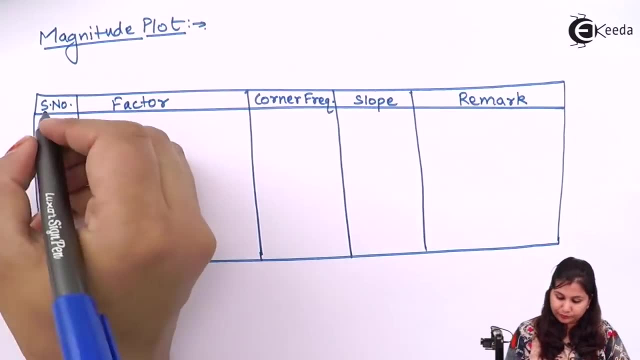 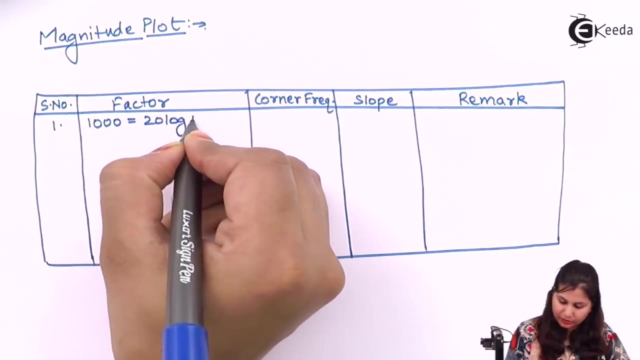 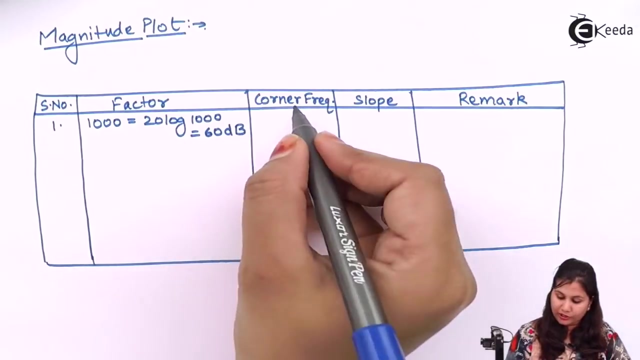 this is our magnitude equation. So the first factor in the transfer function is the constant term 1000,. okay, So first taking the factor 1000, its magnitude will be 20 log 1000.. So we will take the factor 1000 and its value. we have already calculated it is 60 dBs. 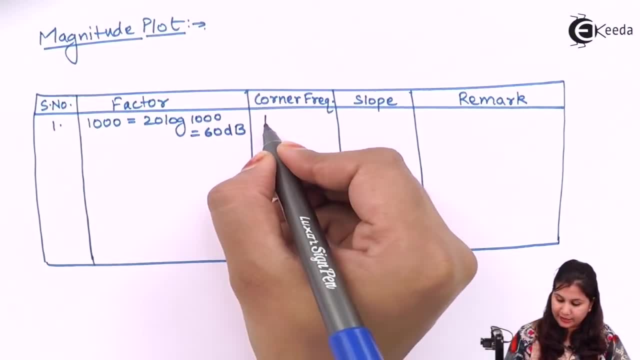 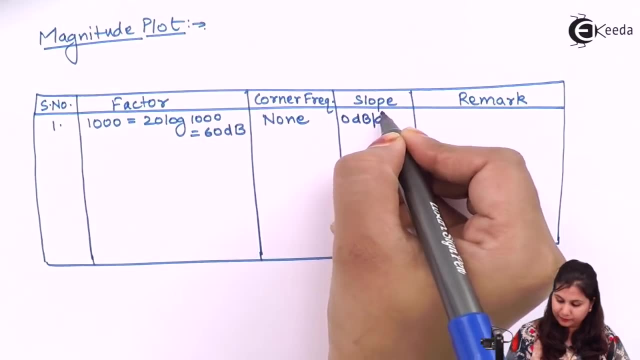 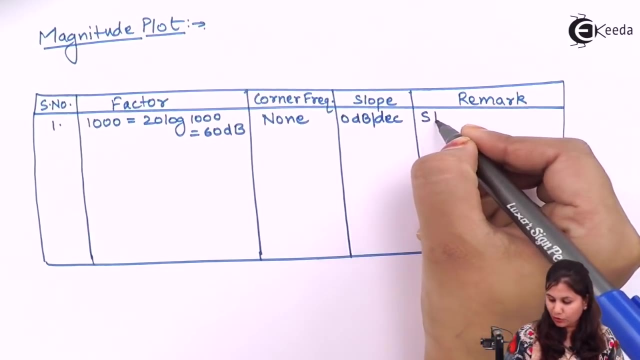 Corner frequency associated with the constant factor is 0, so there is no corner frequency. Slope is 0 dBs per decade. constant term will be having no slope. 0 slope will be there and it will be represented on the boat plot by a straight line having the slope as 0 dBs. 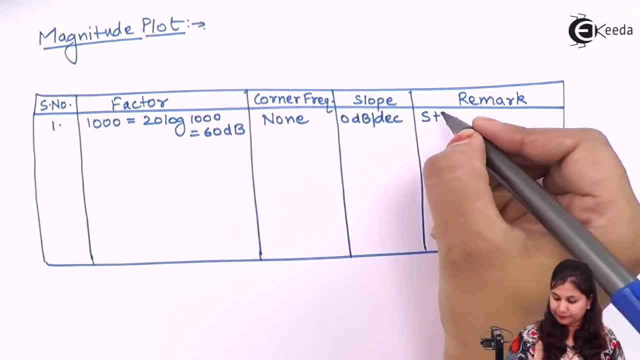 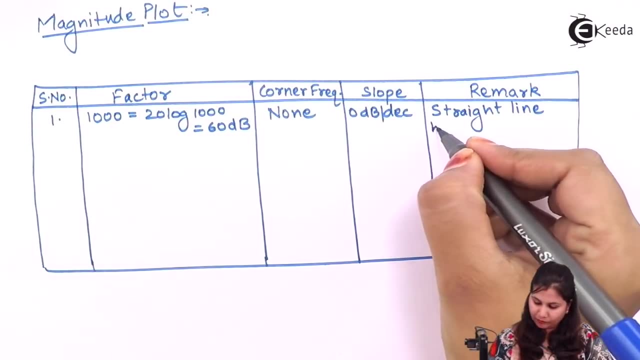 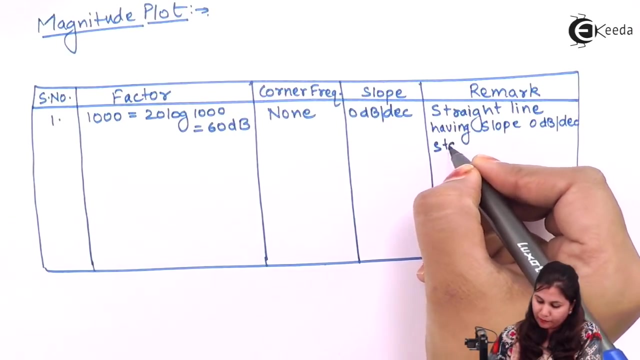 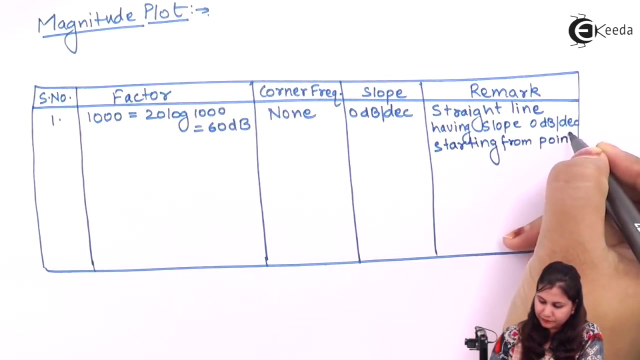 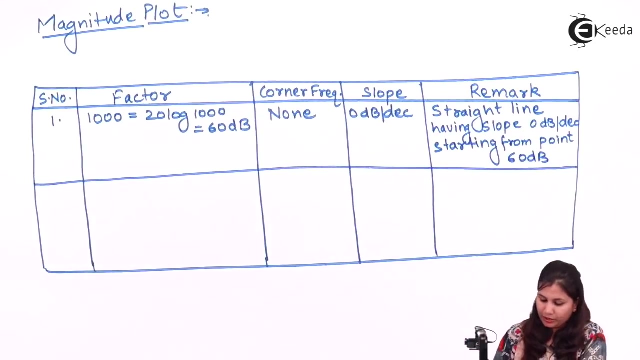 and starting from the point 60 dBs. So this will be a straight line having slope 0 dBs per decade and this will be starting from point 60 dBs. Now, second factor is 1 upon 1 plus 0.1 s and its magnitude is minus 20. log under root. 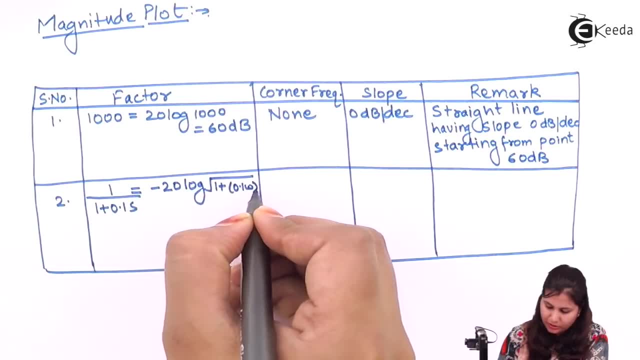 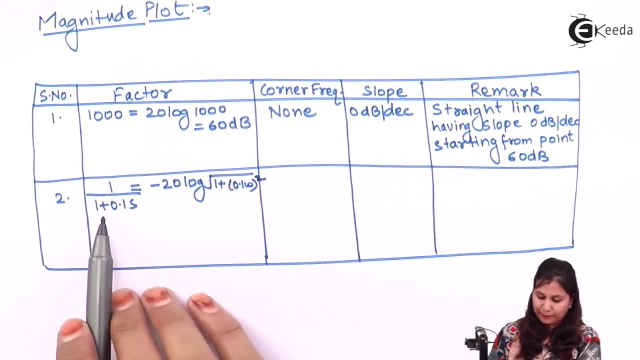 of 1 plus 0.1 omega square. This is the magnitude of this factor. 1 upon 1 plus 0.1 s Corner frequency will be 1 upon omega. so here, this 1 upon the corner frequency, omega will. 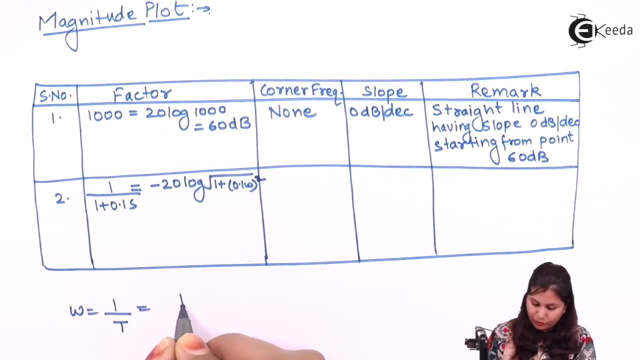 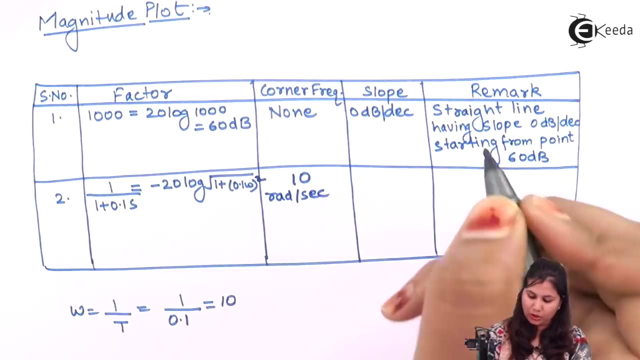 be 1 upon t. Here time constant is what 0.1,, so 1 upon 0.1,, it will be 10.. So corner frequency is 10 radians per second. Slope, Slope, Slope. 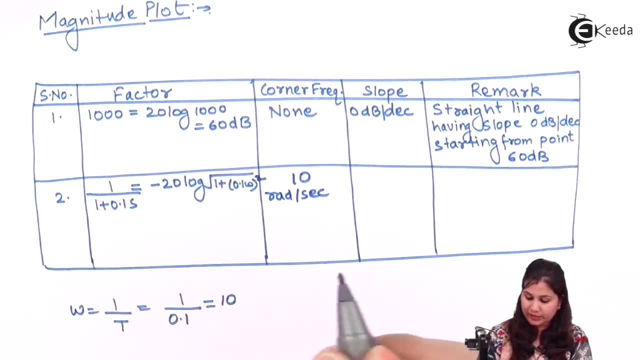 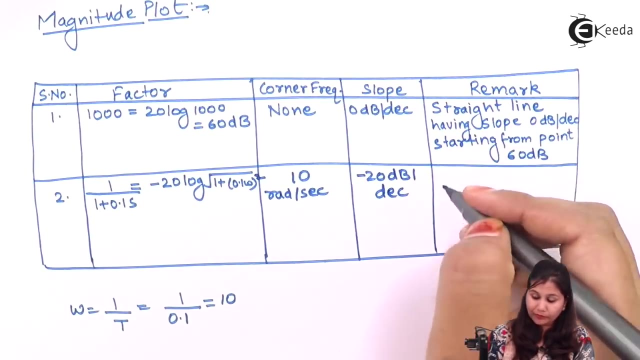 The slope associated with this first order factor is minus 20 dBs per decade Because it is a first order factor. so the slope will be minus 20 dBs per decade and it can be represented on the boat plot by a straight line which is having the slope minus 20 dBs. 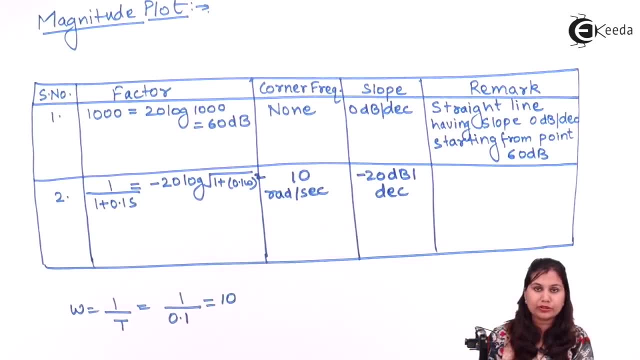 per decade, and starting from the frequency, omega equals to 10.. Okay, Okay, Okay. So this is the second factor. Now, third factor is 10, so 2 upon 2 s, again 2 to the last, 3 is a 3 too, so 0 and 0 equal to 6, so 4 times this is equal to 10. 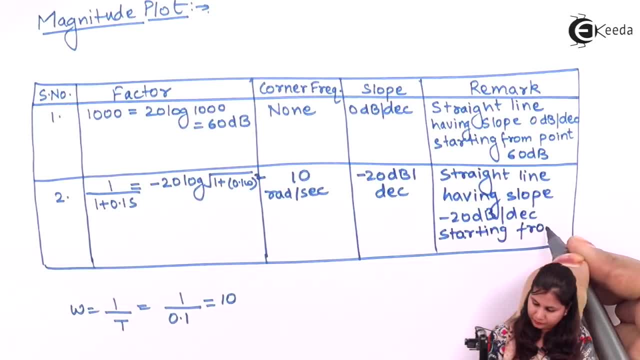 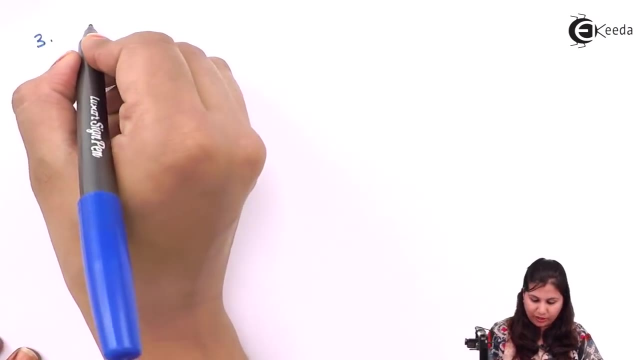 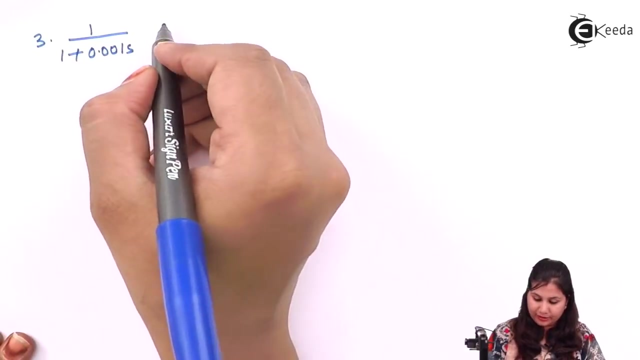 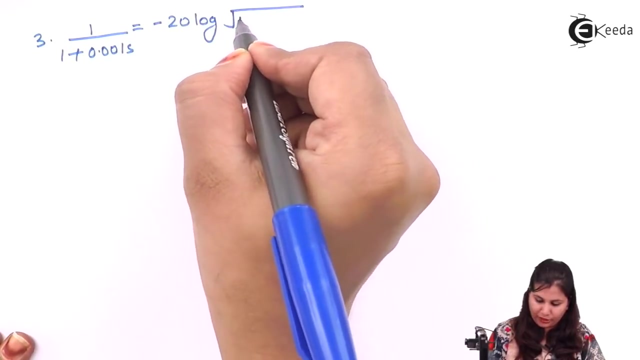 to 3.. It cannot be a partial coprime, which is a partial number. Now, here positive is 7 and negative is 1 upon 2 times, then minus 2 times, and a decline is 0.2.. third factor is 1 upon 1 plus 0.001 s and its magnitude will be minus 20 log under root of 1. 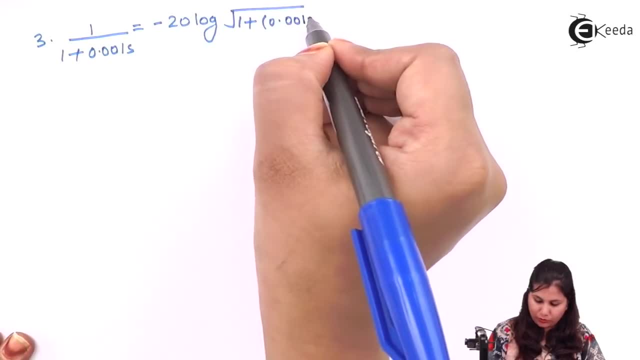 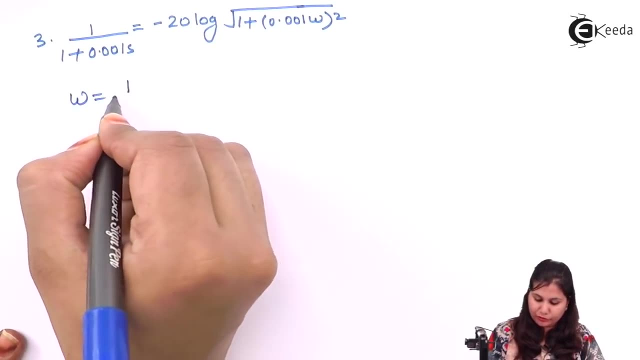 plus 0.001 omega square. So this is the magnitude Corner frequency will be here. omega equals to 1 by t, So 1 by here. time constant is 0.001.. So the frequency will come out to be 1000 radians per. 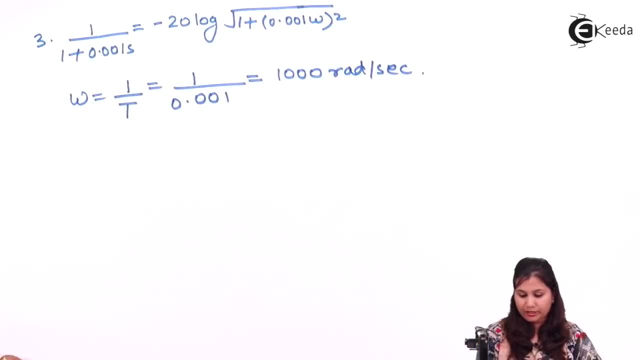 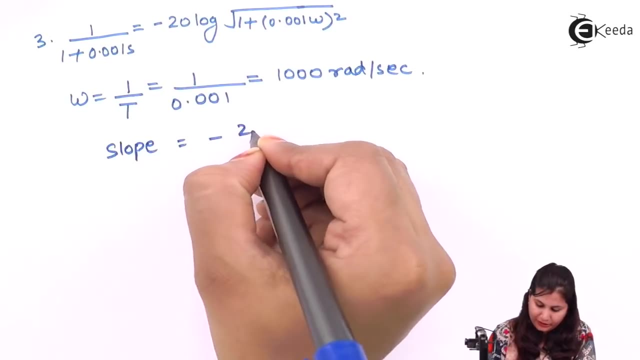 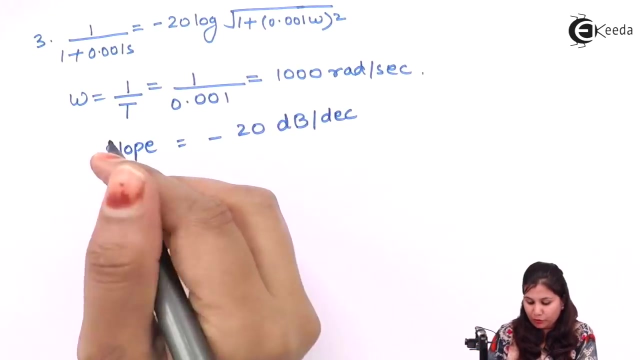 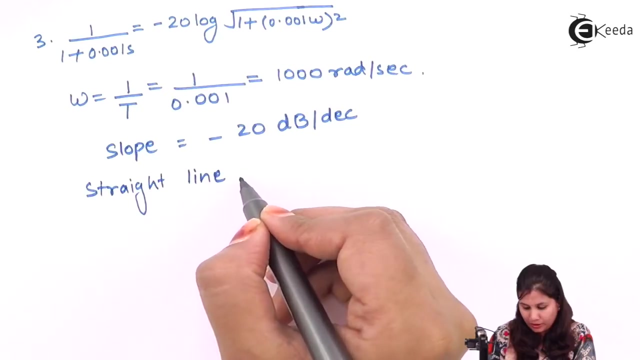 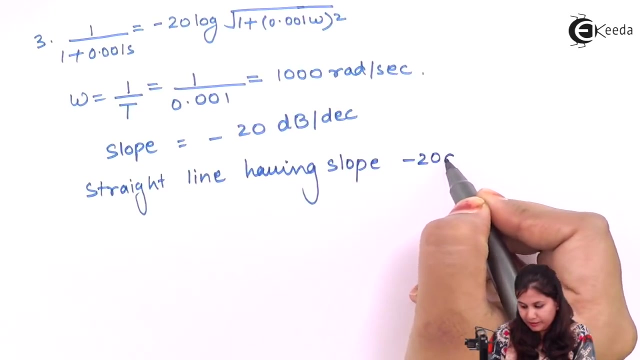 second: Okay Now this factor is a first order factor, So slope will be minus 20 dBs per decade. And how we can represent this on the board plot, it will be a straight line having slope minus 20 dB per decade starting from. 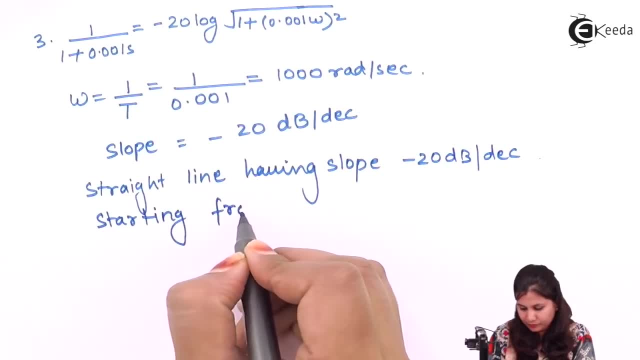 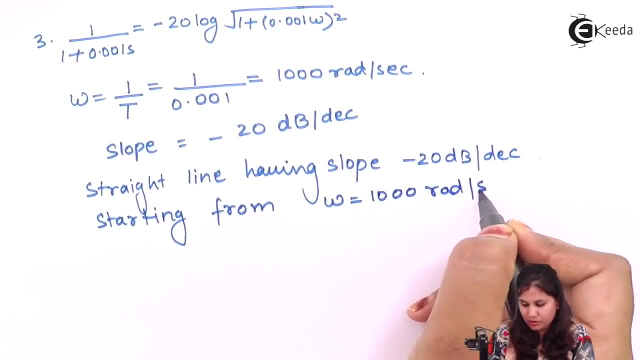 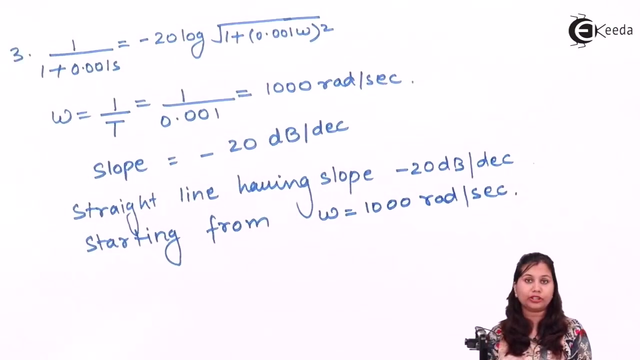 omega equals to 1000 radians per second and is starting from the corner frequency. So we have considered all the three factors in the transfer function and we have seen that how they can be represented in the magnitude plot. Now let's form the table for the phase. plot For phase. 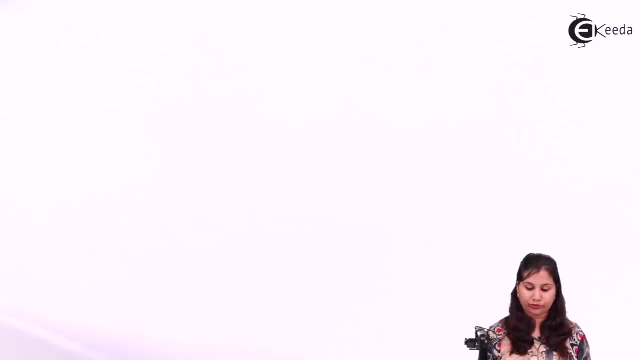 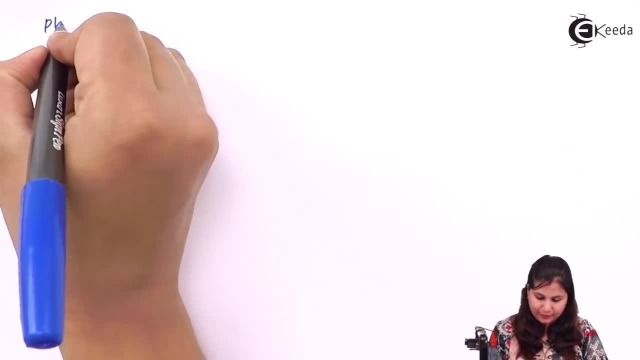 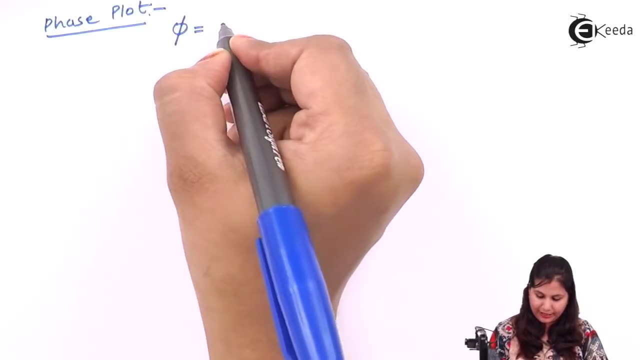 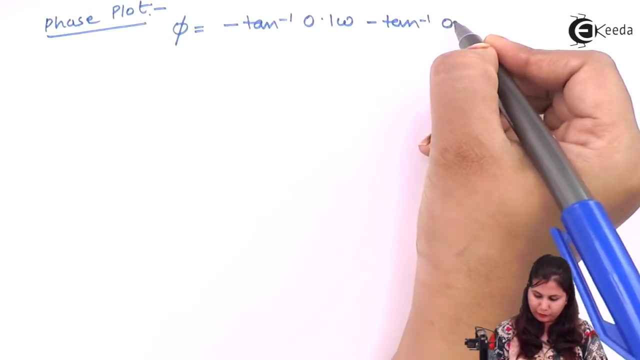 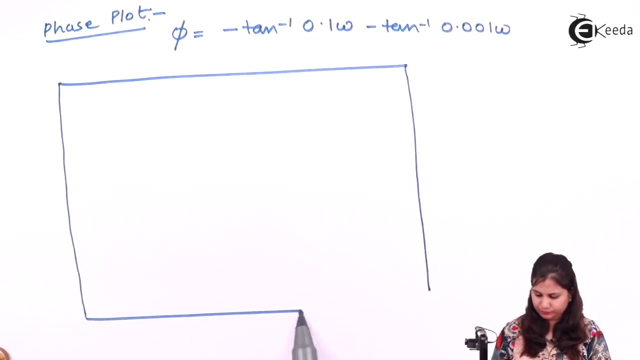 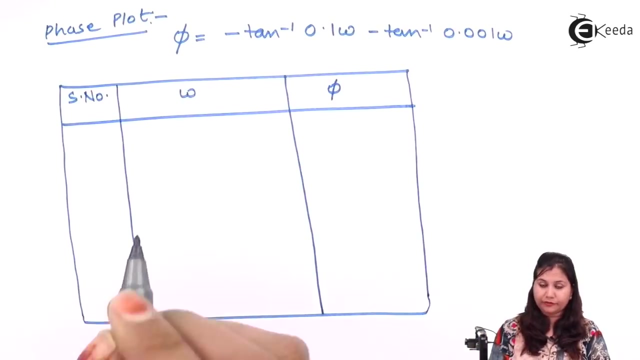 phase angle phi. So phase angle is we have the phase equation phi as minus tan, inverse of 0.1 omega, minus tan, inverse of 0.001 omega. So let's form the table. The first this: here we are going to take different values of omega and then we can calculate the value. 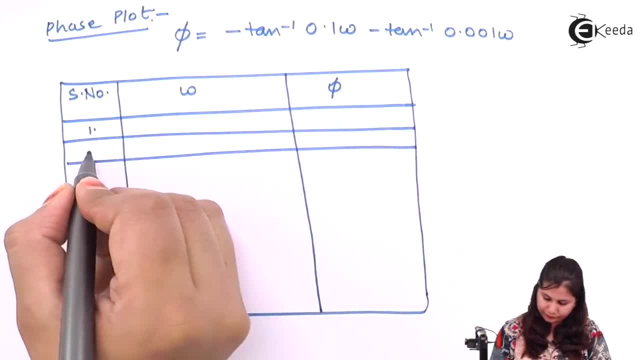 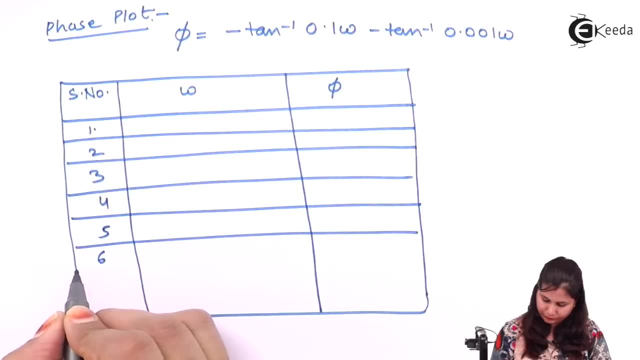 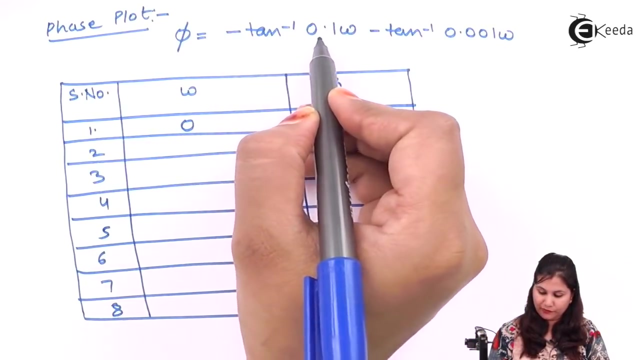 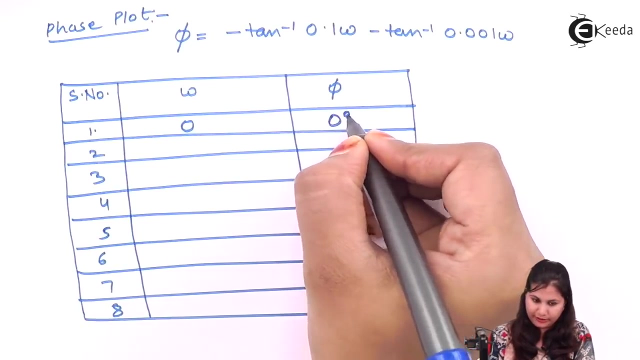 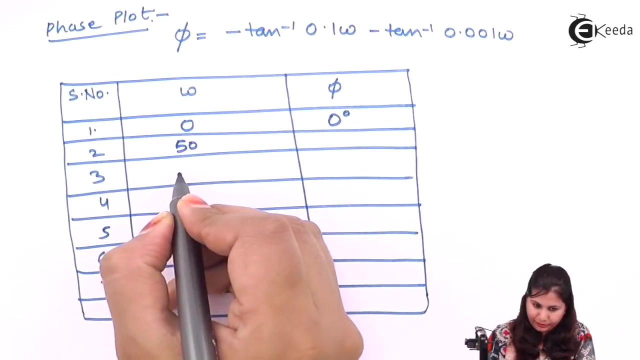 of phi. Let's take the first value of Omega as 0, so putting here Omega equals to 0, Omega equals to 0, so it will become minus tan inverse of 0, minus tan inverse of 0 and tan inverse of 0 degrees. 0 is 0 degrees. ok, now for Omega equals to fifty hundred five hundred. 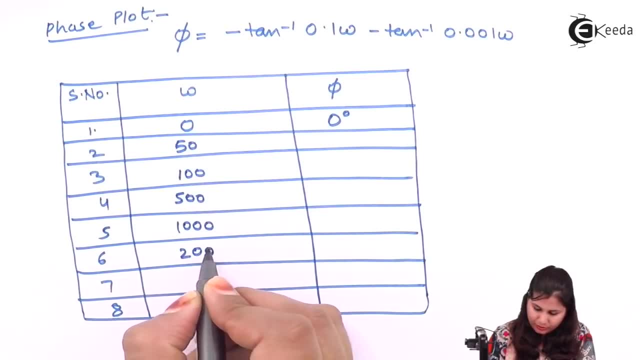 thousand, two thousand eight thousand and infinity. we have two different values of Omega, depending upon what range of frequencies we are getting in the magnitude plot. we were getting the corner. frequency of omega is 0 and the magnitude of omega is 0, so now what will happen? 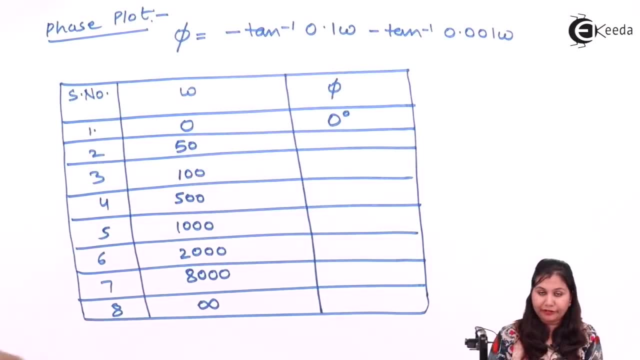 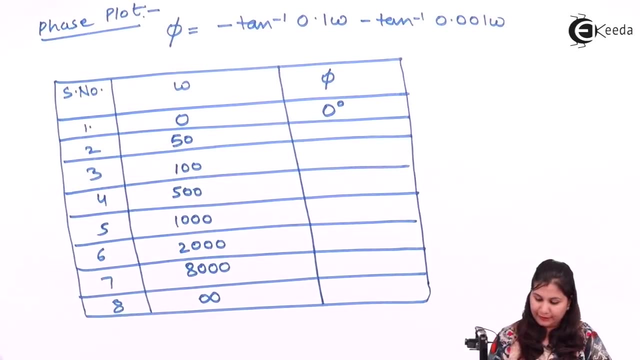 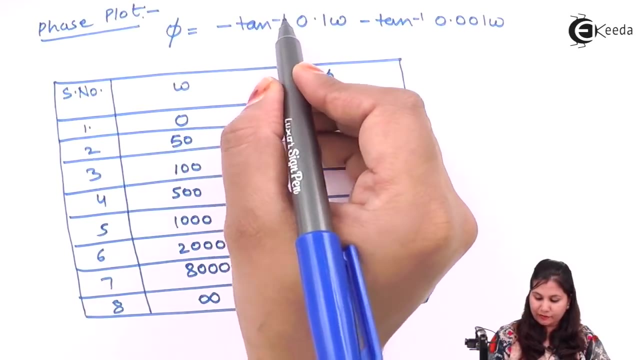 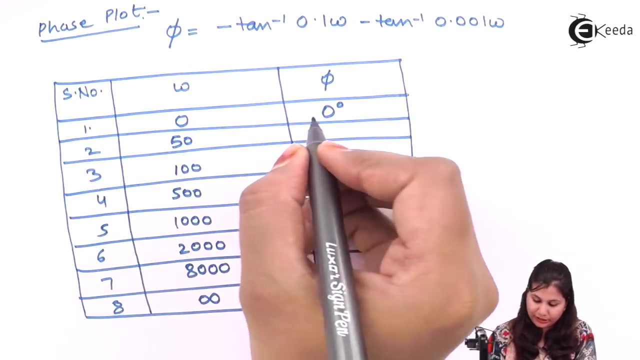 frequency as 1000 and this 50, 10 we are getting. so let's take the multiples of 10 here as the frequency scale. so for omega equals to 50, put here 50, here also 50, so it will become minus tan inverse of 0.1 into 50 and minus tan inverse of 0.001 into 50. let's calculate so the 5 will be. 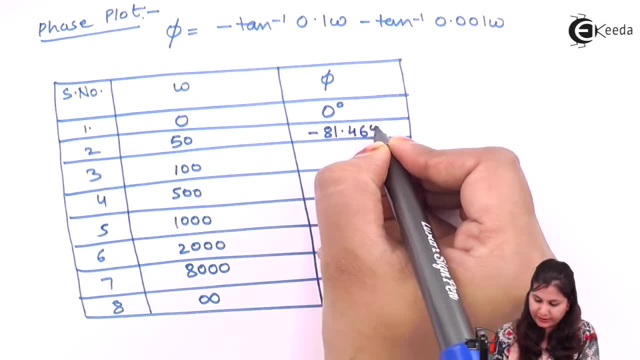 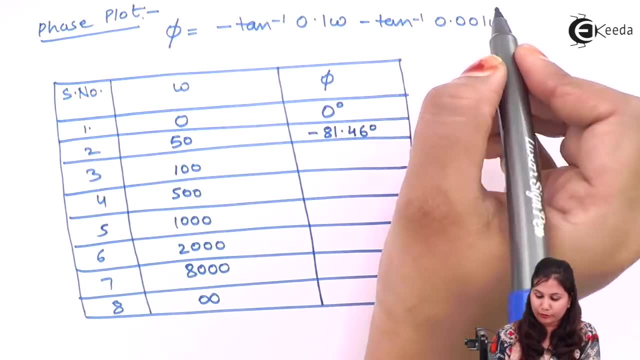 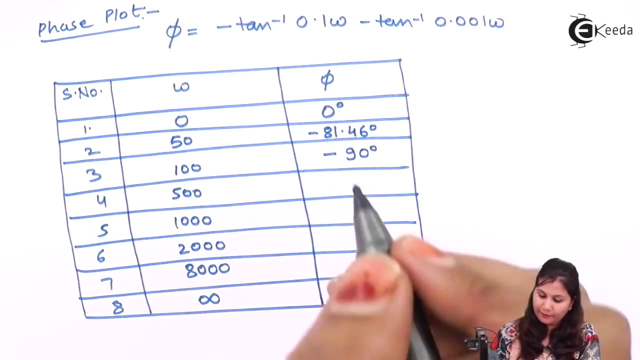 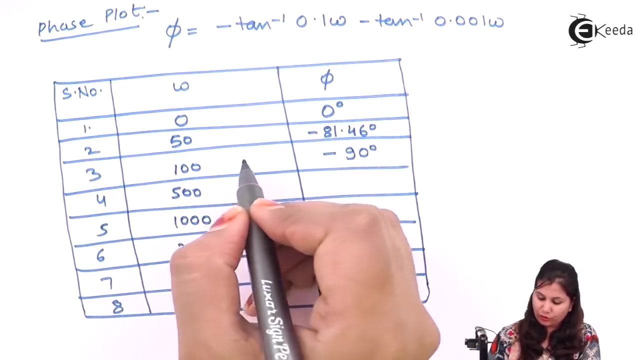 it will come out to be minus 81.46 degrees, for omega equals to 100 here, 100 here also put this, omega equals to 100, so the value of 5 will come out to be minus 90 degrees. okay, because it will be 0.1 into 100. so it will be tan inverse of 10, and then here also, if we solve this, it will come. 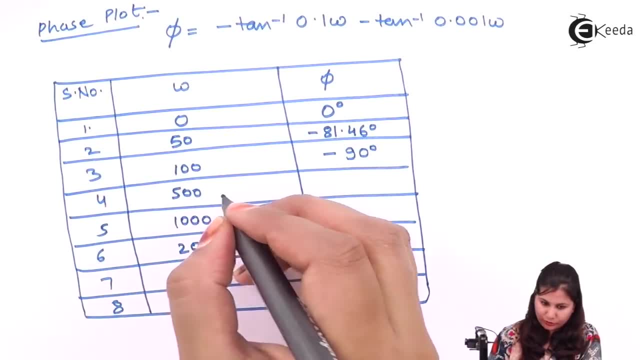 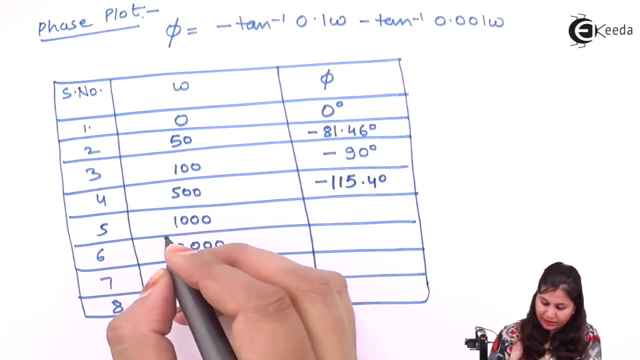 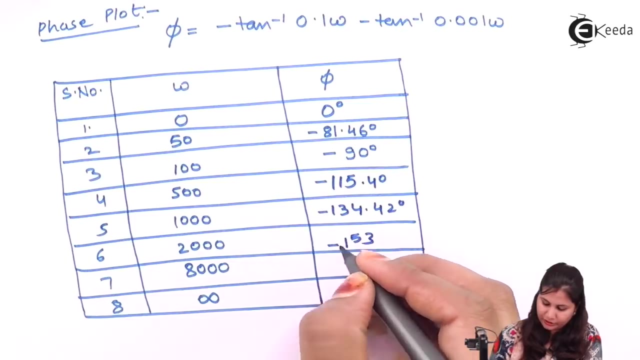 out to be minus 90 degree, then omega equals to 500. the phase angle will be minus 115.4 degrees, For omega equals 2000. similarly we are going to calculate for 2000,. 8000 and infinity. It will be minus tan, inverse of infinity minus. 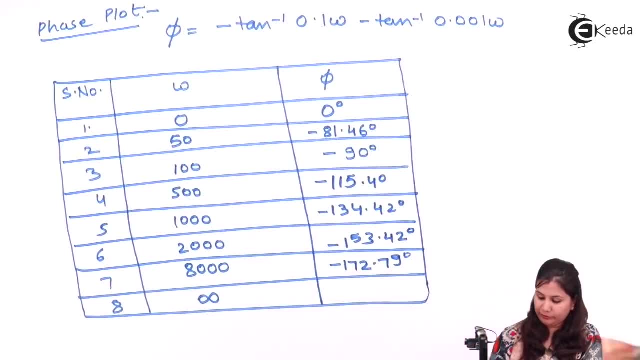 tan, inverse of infinity. So minus 90, minus 90 it will be minus 180 degrees. So for different values of omega, we have calculated the phase angle 5 and we have obtained both the tables for magnitude plot also, and for the phase plot also. Now we are going to plot both these. 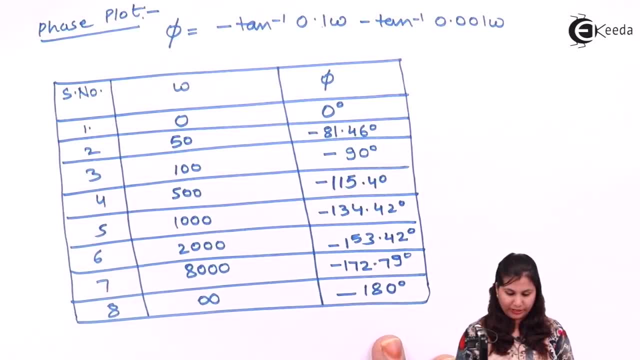 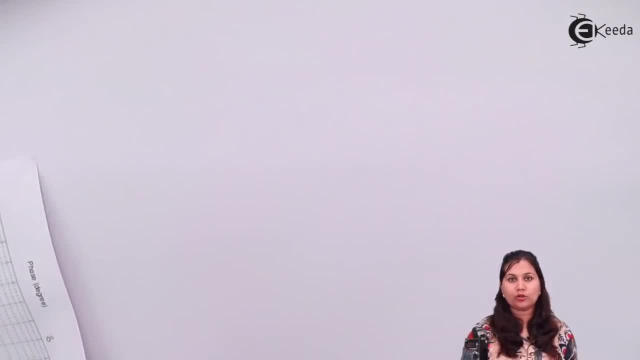 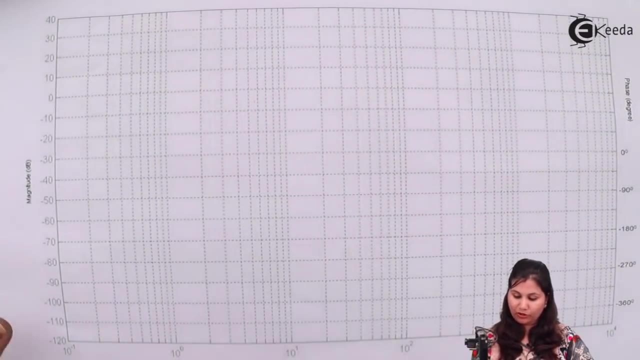 plots on the board plot. So let's see how we can draw The board plot. it is a logarithmic plot. So for sketching the board plot we are going to use a semi-log graph and on this semi-log graph it is having logarithmic scale. You can see that on the 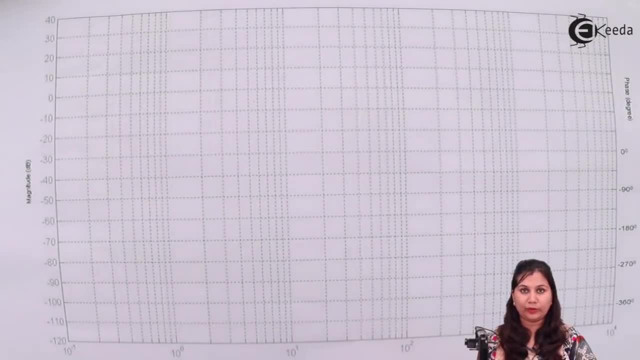 x-axis we are going to represent the frequency and the scale is like tan inverse of 1, that is, 10 raised to the power minus 1,, 10 raised to the power 0, 10 raised to the power 1,, 10 raised to the power 2,, 10 raised to the power 3,, 10 raised to the power 4.. 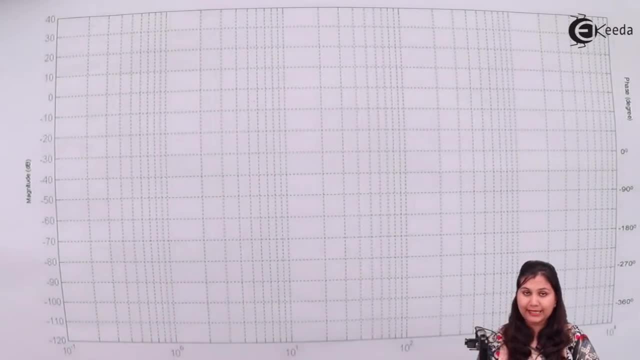 So this x-axis, it is having the scale division as the power of 10.. And power of 10 means per decade, Decade term we have used because per decade, per 100 divisions, how the value is changing, because we are using the power of 10 as the x-axis scale range. Now on the y-axis. both sides. we have a x-axis written here, And if we write a piece of 10 on the y-axis then we have a 10.. So the difference will be that total number of degrees divided by n, when it 윩, is greater than 1.. So this x-axis that is to be multiplied by cũng. 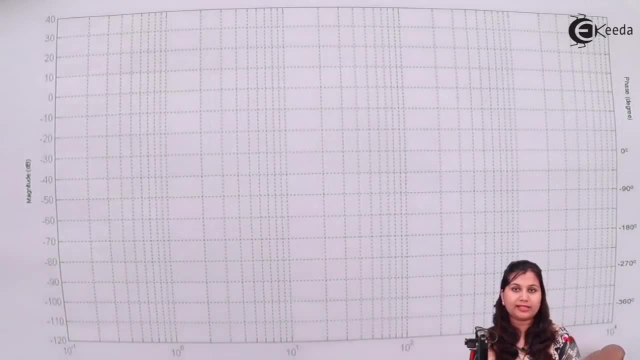 q vontade cm gain, and of course that is 10 per x-axis and number of degrees. we have to write this in can only in a lot of gotta know means if P x is greater than 10, while where this sides, on the left hand side, we are going to use the magnitude, we are going to plot the magnitude. 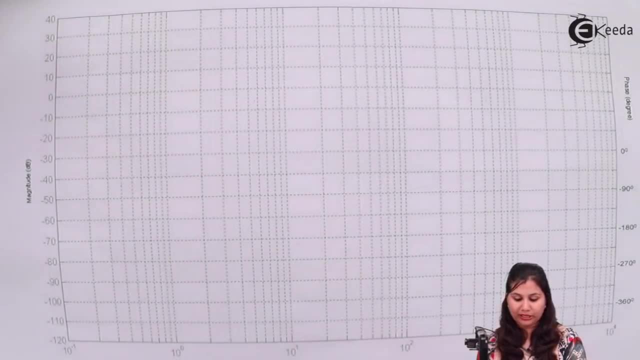 here we are going to use 0, 10, 20, 30, 40 and then minus 10, minus 20, minus 30. this is the scale range. we can change the scale range or the position of 0 according to our question. so on left hand side, 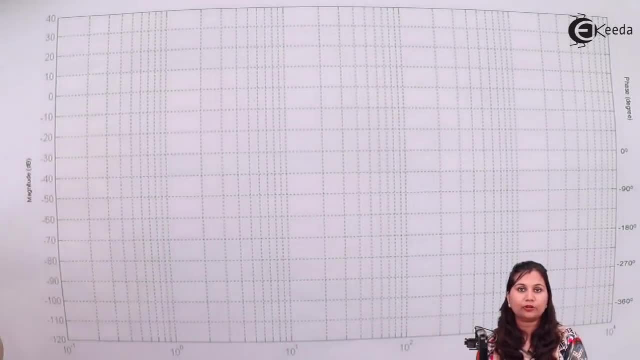 we are going to use the magnitude and on the right hand side we are going to plot the phase. that is, we are going to use this scale for plotting the phase plot. here we are having the phase angles like 0 degrees, 80 minus 90, minus 180, minus 270, minus 360. so upper part we are 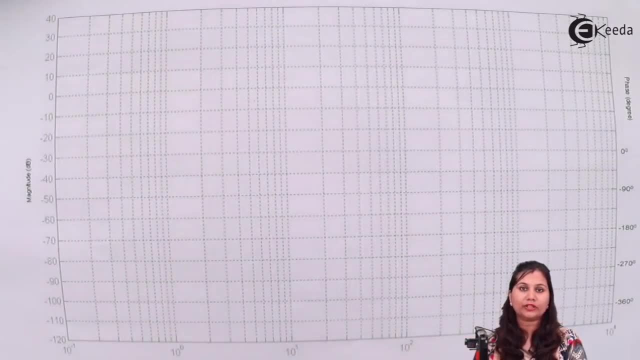 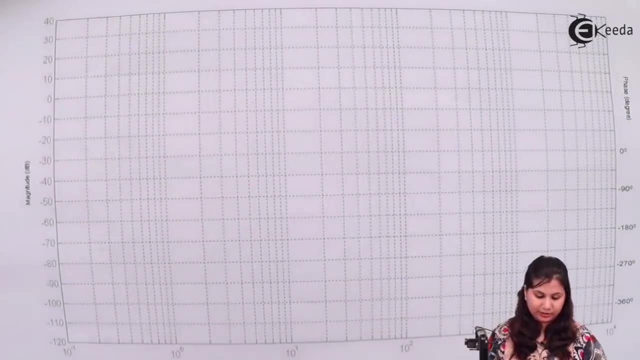 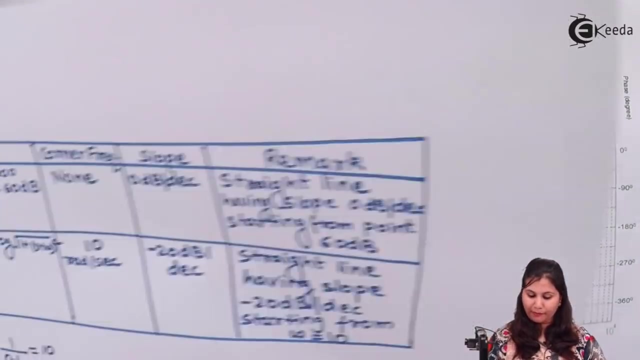 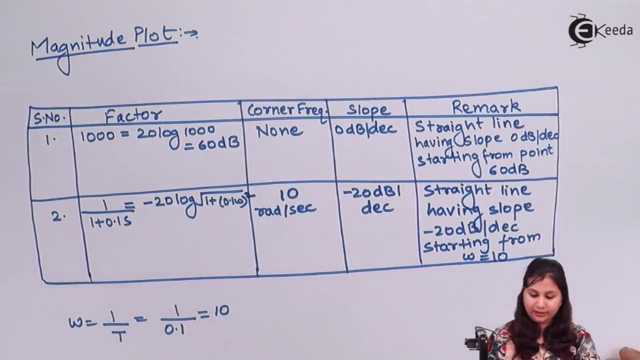 going to plot the magnitude and on the lower part, we are going to plot the phase angle of the transfer function. okay, so let's see our table for the magnitude, what we have got here. okay, for magnitude, we are having the first factor as 1000 and the magnitude of this 1000 factor is: 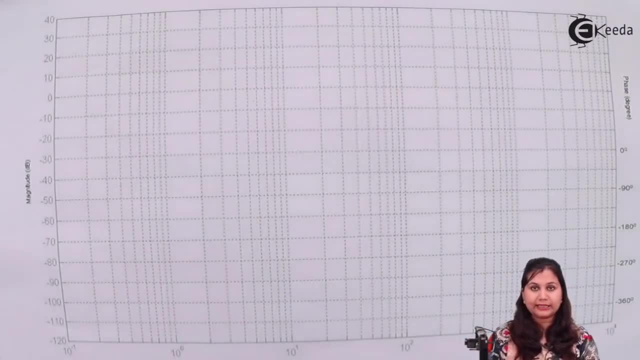 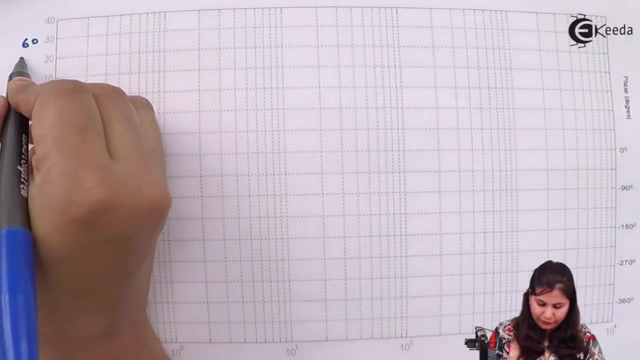 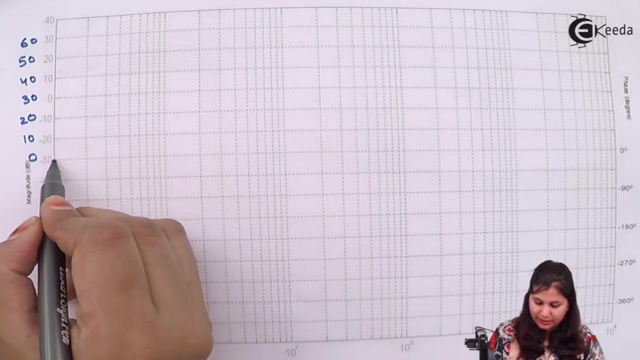 60 dbs. so you can see that in this board plot we are not having 60, so we can change this scale according to our question. mark this as 60, 50, 40, 30, 20, 10 zeros. so this is a 0 db line. okay, mark this line. 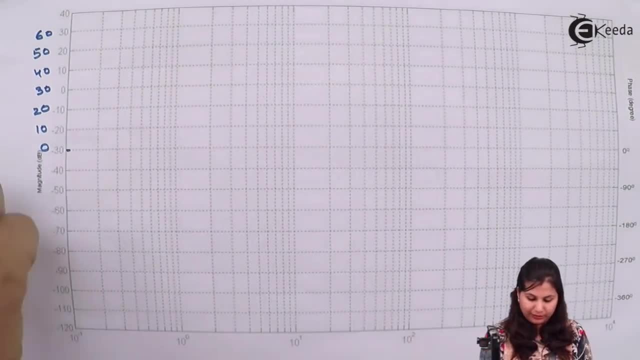 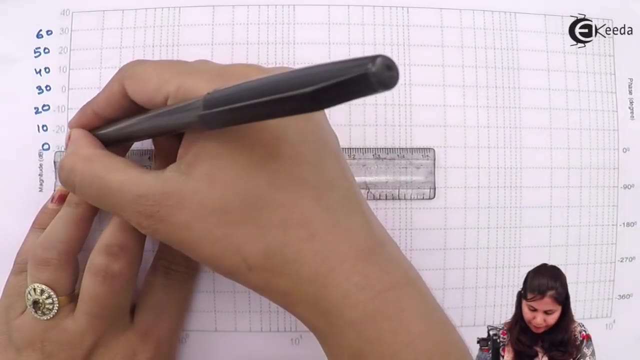 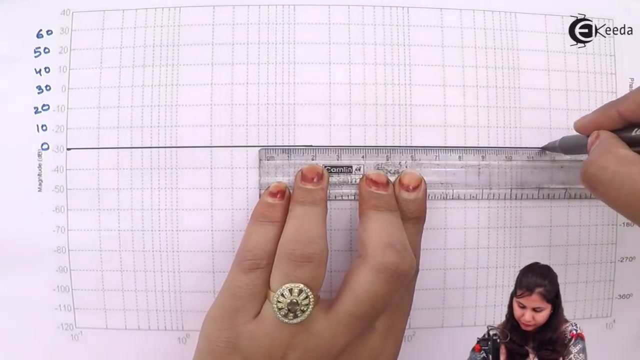 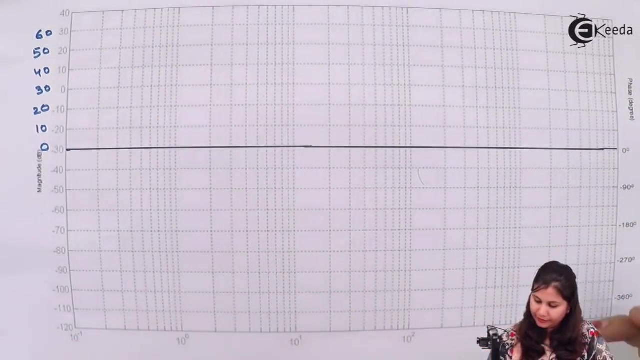 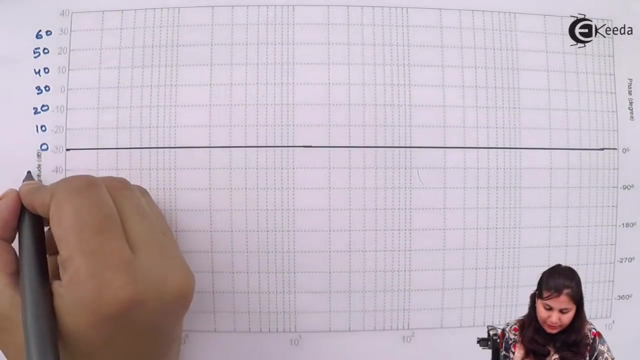 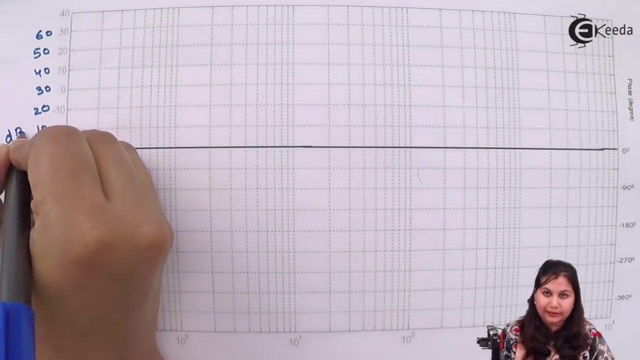 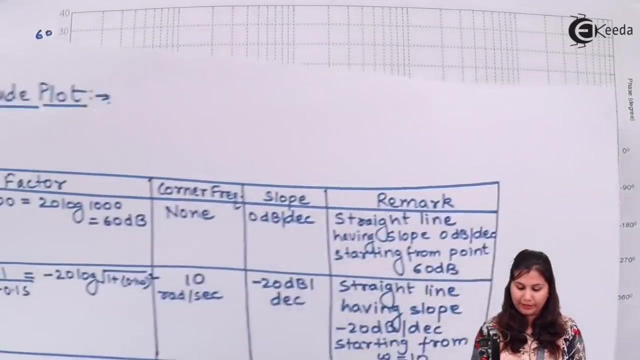 so let's mark this line 0, db line. okay, and here we are having zeros, minus 90, minus 180. for that phase angle, this will be minus 10 minus 20, minus 30. okay, this is in dbs, the magnitude, okay, so first factor, that is 1000. it is having the 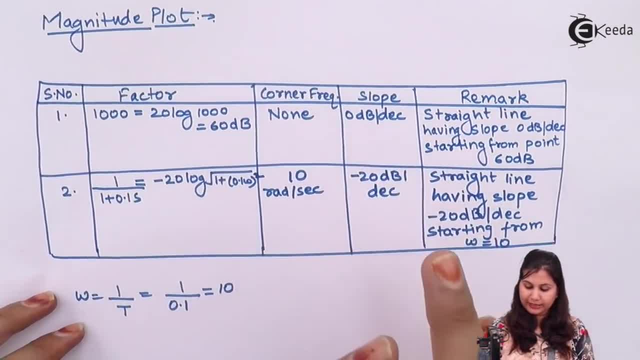 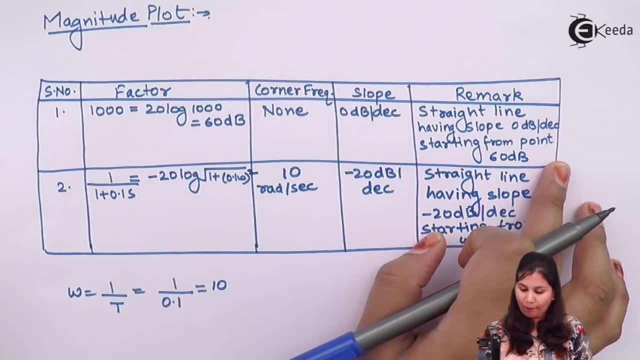 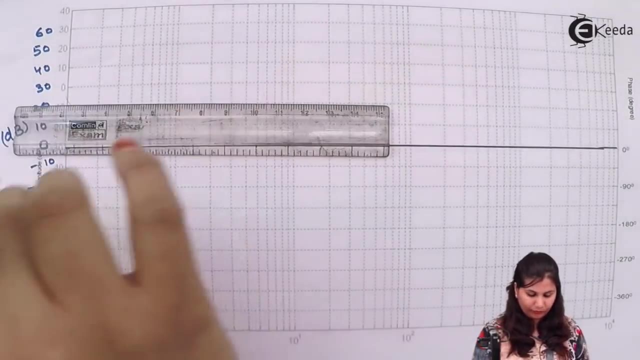 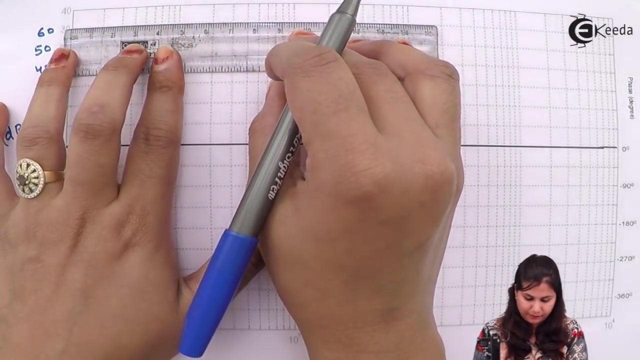 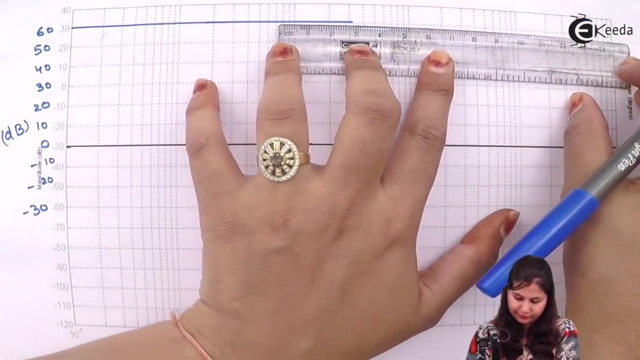 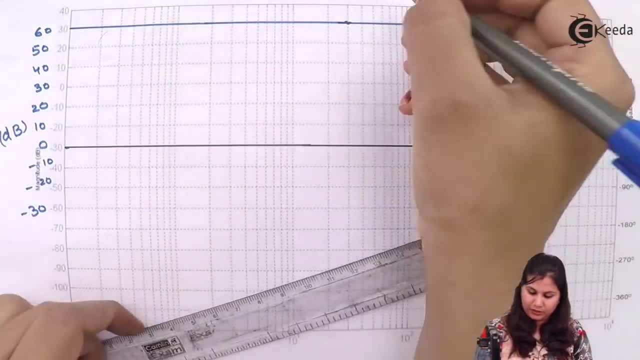 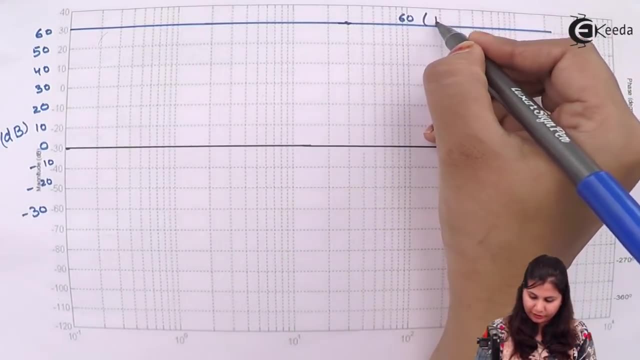 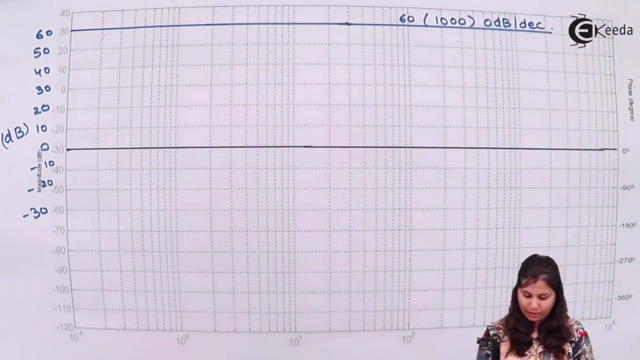 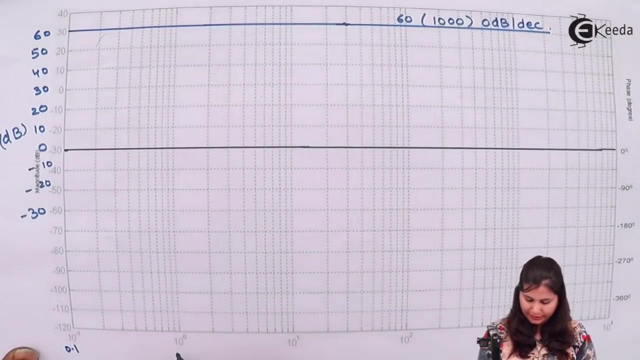 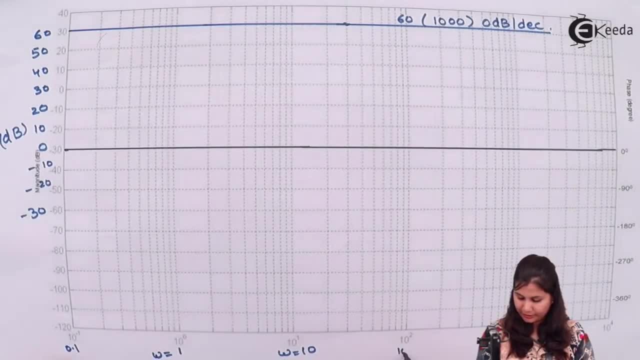 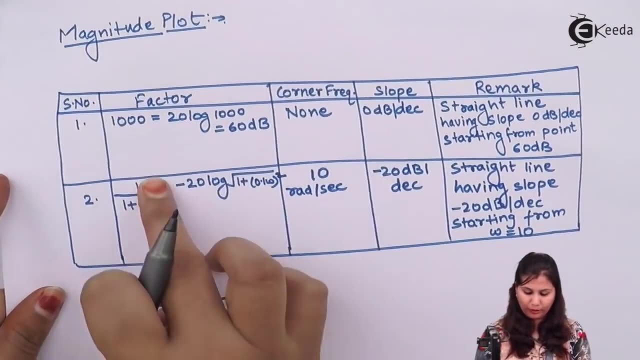 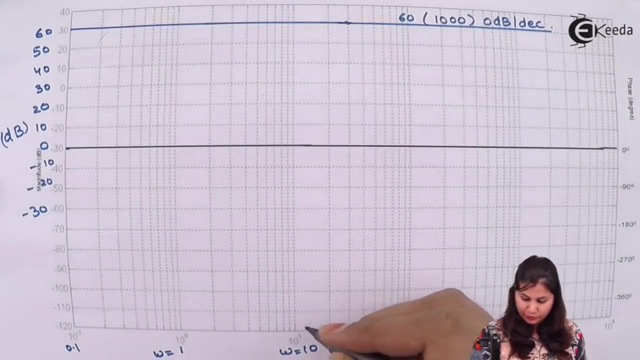 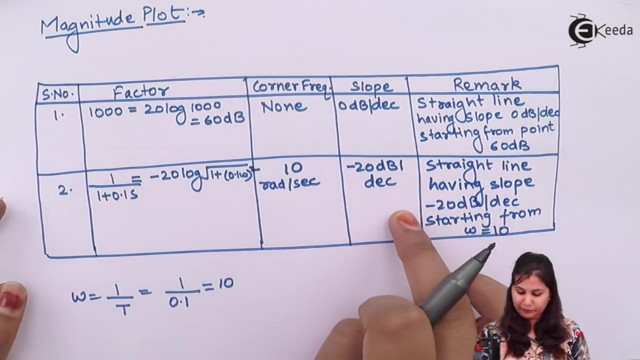 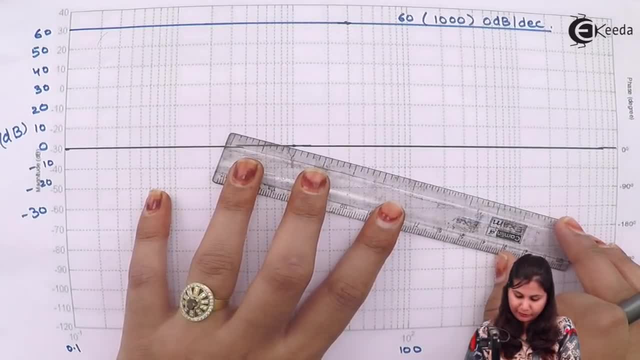 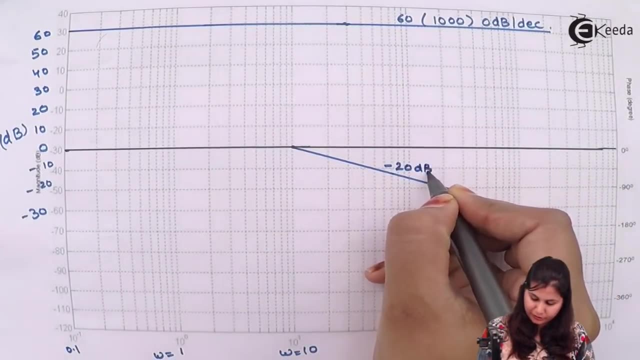 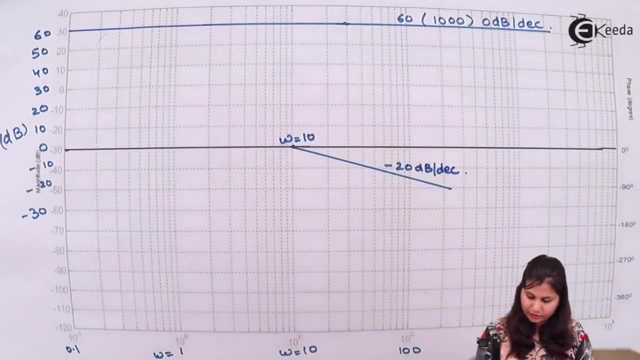 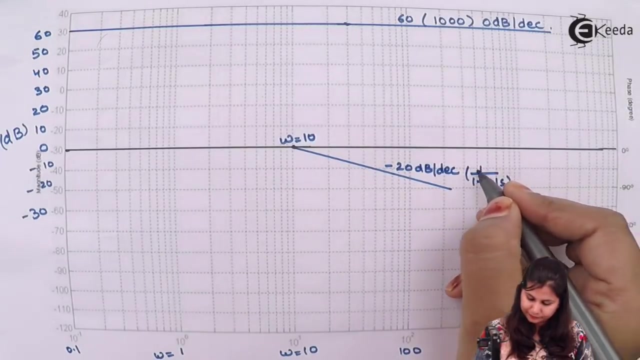 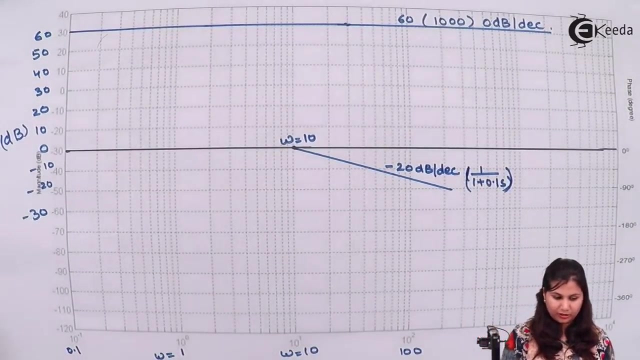 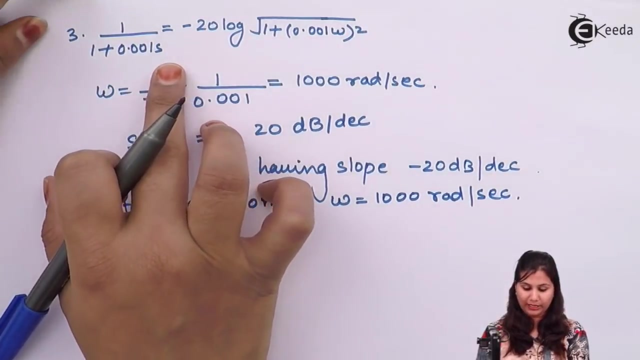 with slope minus 20 dB per decade. draw a line. So this is minus 20 dB per decade and this is omega. equals to 10 due to the factor 1 upon 1 plus 0.1 S. Now third factor is omega. we have third factor as 1 upon 1 plus 0.001 S and its corner. 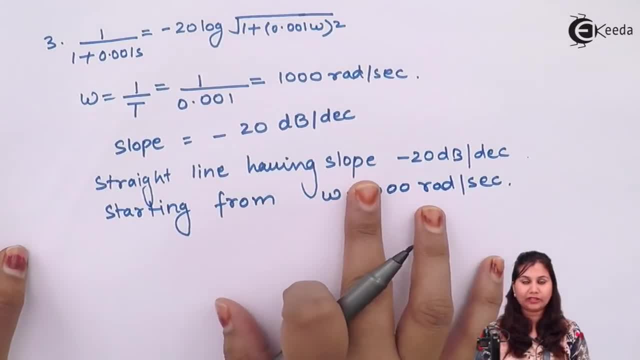 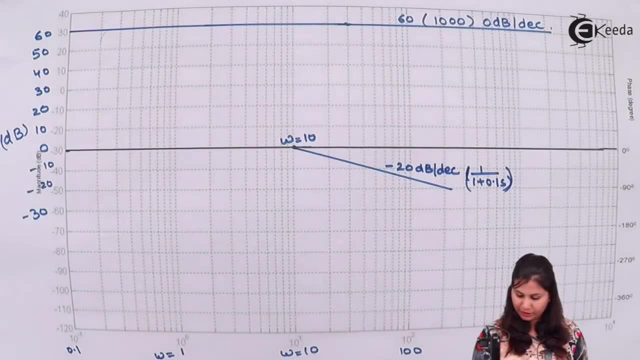 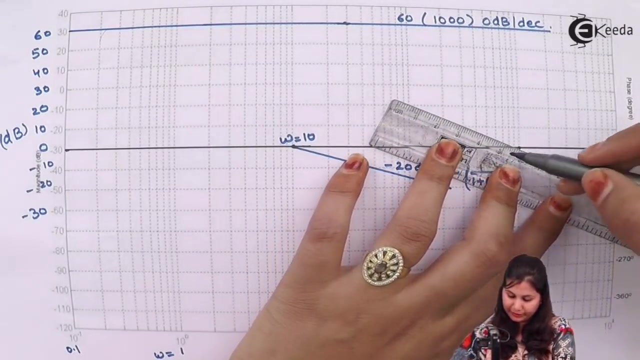 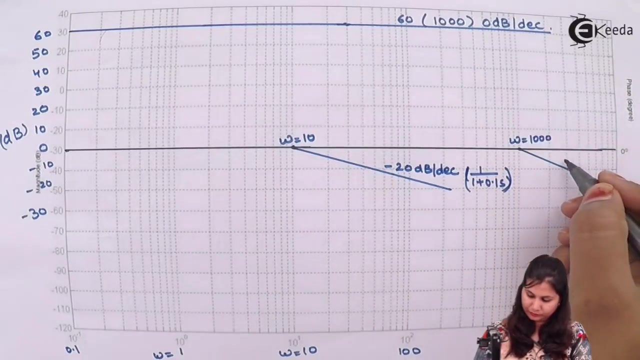 frequency is 1000. So it will be a straight line having the slope minus 20 dB per decade, starting from omega equals to 1000.. So, starting from omega equals to 1000, here We have a line having the slope minus 20 dB per decade due to the factor 1 upon 1 plus 0.001 S. 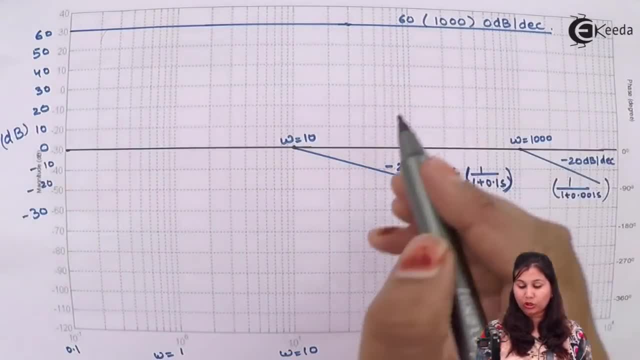 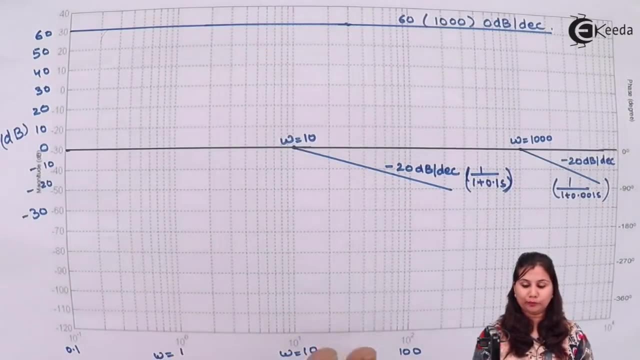 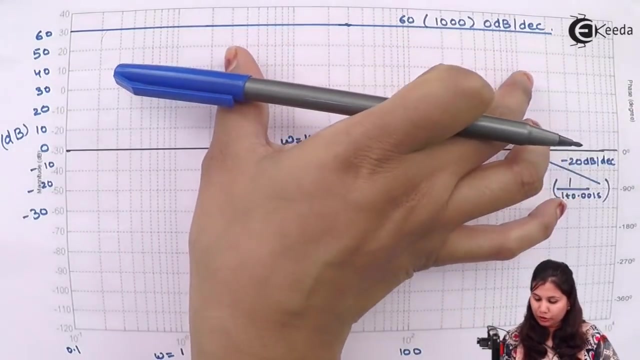 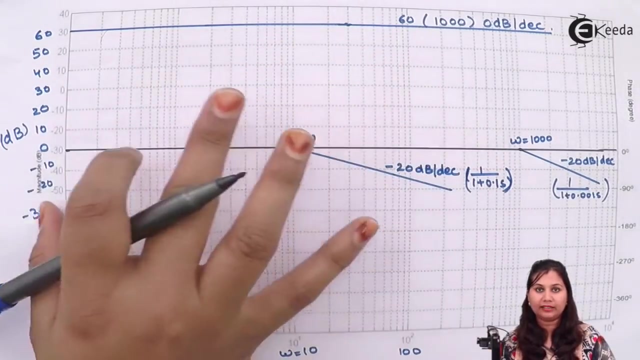 So we have represented all the three factors on the magnitude plot. Now to draw the resultant magnitude plot we have to add up all these individual plots, That is, individual plot of the constant term due to this first order factors. So all these three plots they are going to add up so that we can get the resultant magnitude plot. 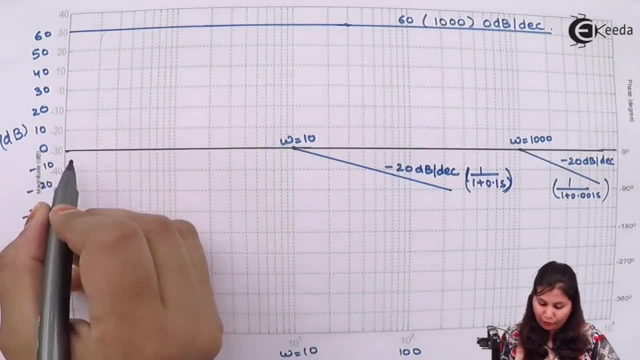 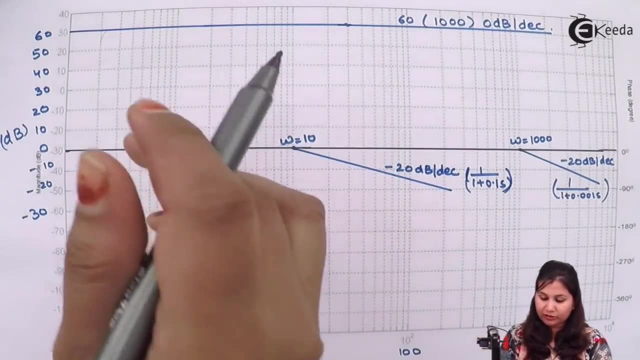 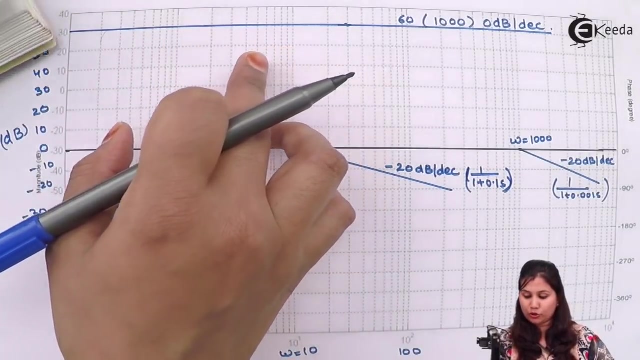 So let's Add here from starting from the frequency: omega equals to 0.1 to omega equals to 10. We are having the slope as 0 dB and the magnitude is 60 and the slope is 0 dB, So it will be a straight line. 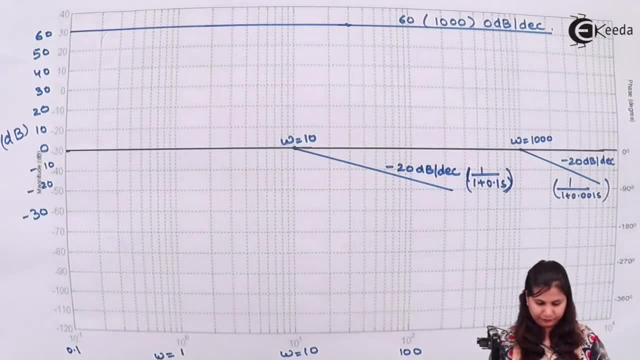 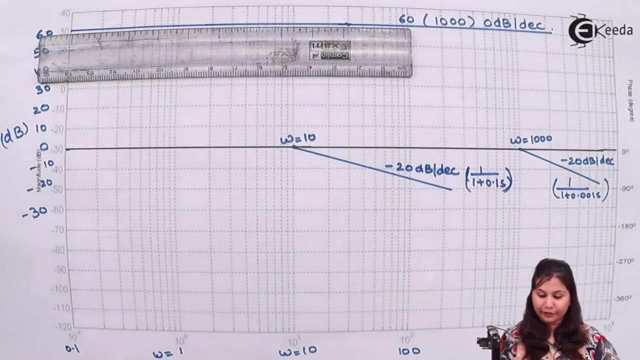 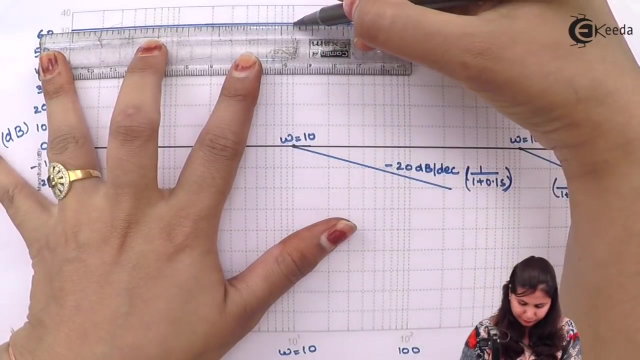 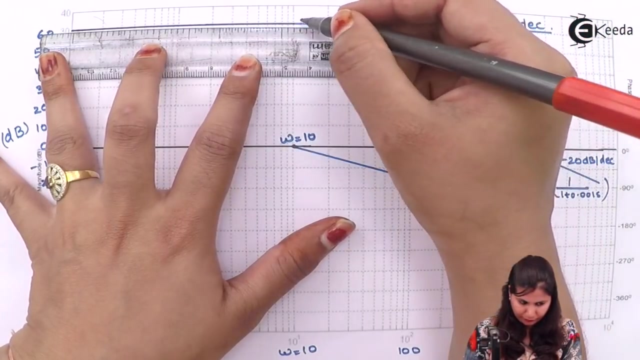 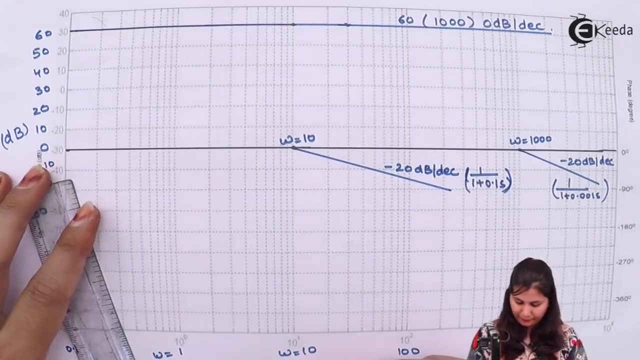 Okay, Up till now, that is omega equals to 10.. Our magnitude plot will be a straight line Now from omega equals to 10, it will be minus 20 dB per decade due to this factor. So it is going to add up. 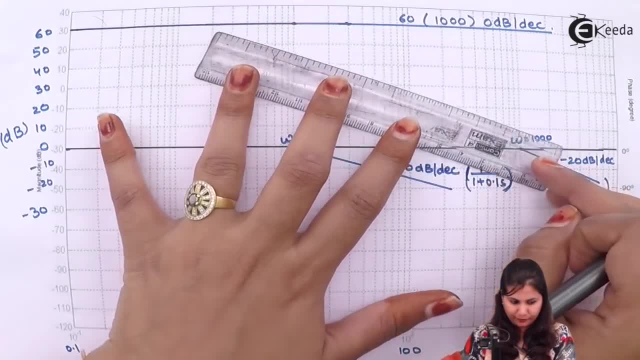 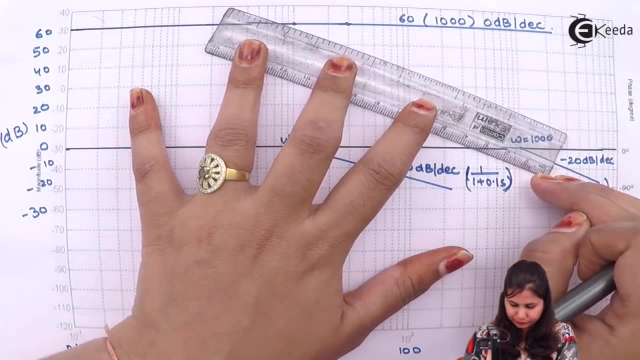 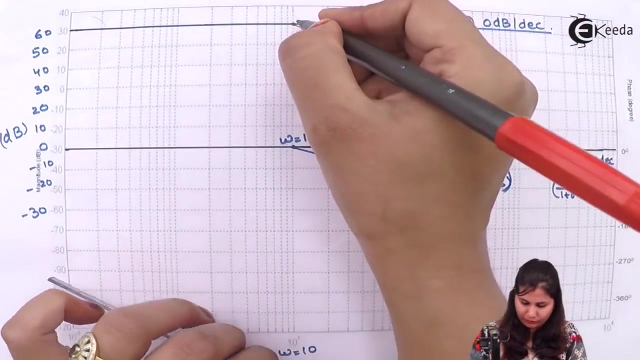 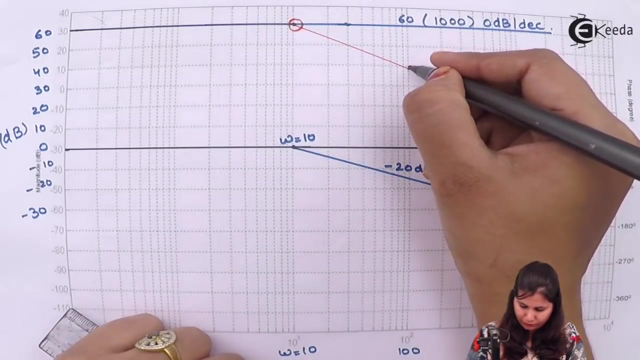 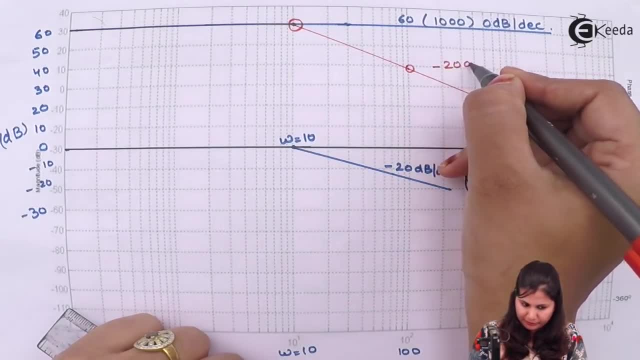 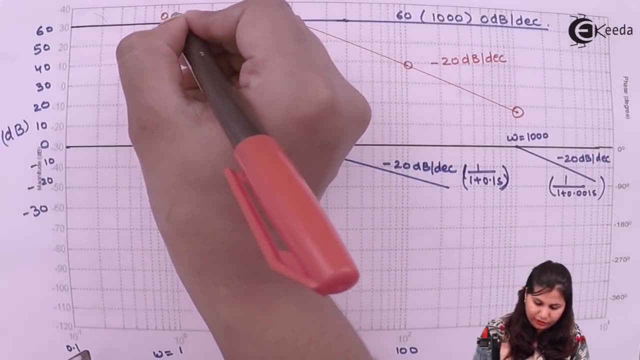 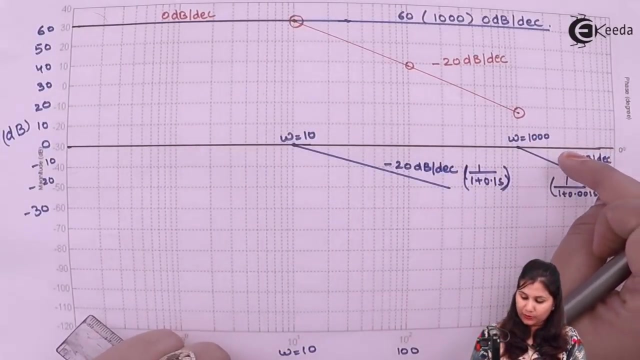 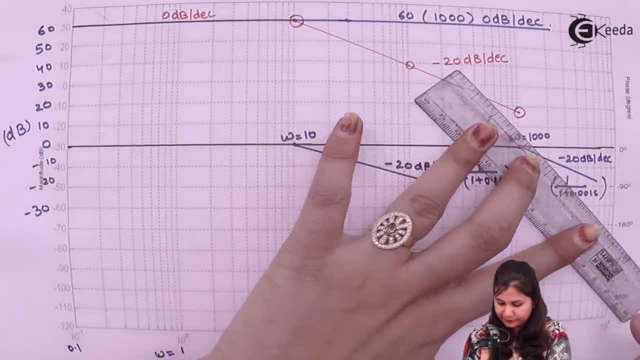 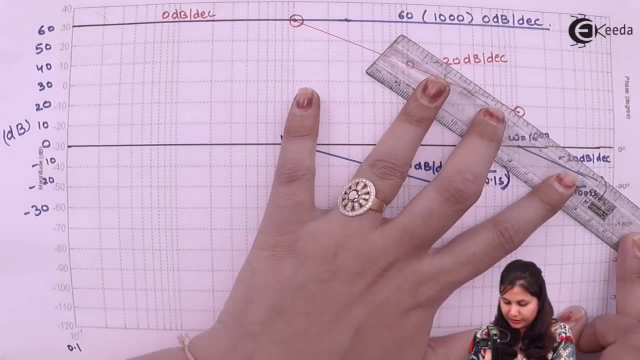 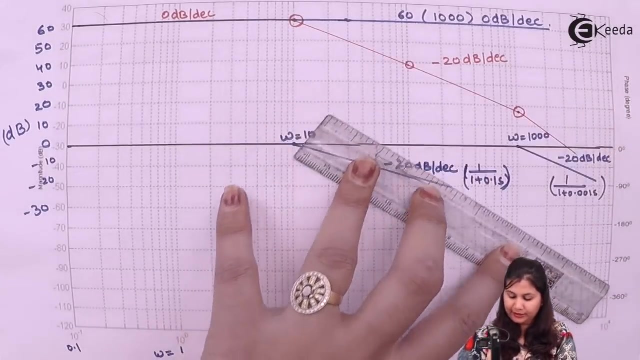 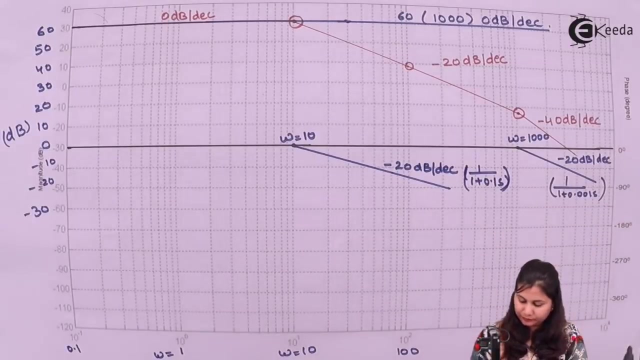 add up. so here we are going to add this: this was minus 20, so minus 40. minus 20, minus 20, it will be minus 40. so it is going to be like this: this is minus 40 dB per decade. so this is our complete magnitude plot. now phase plot we have to draw. so for phase plot, 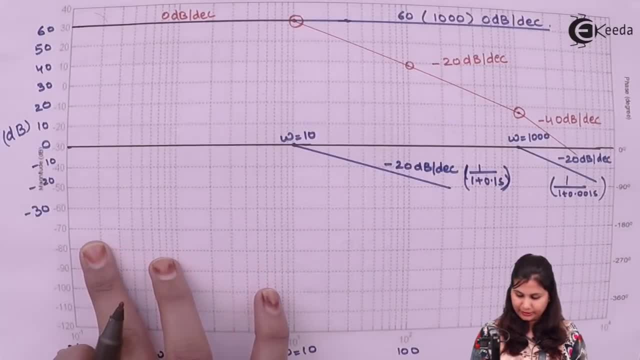 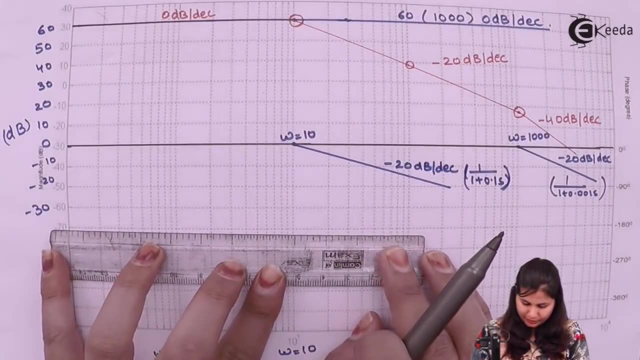 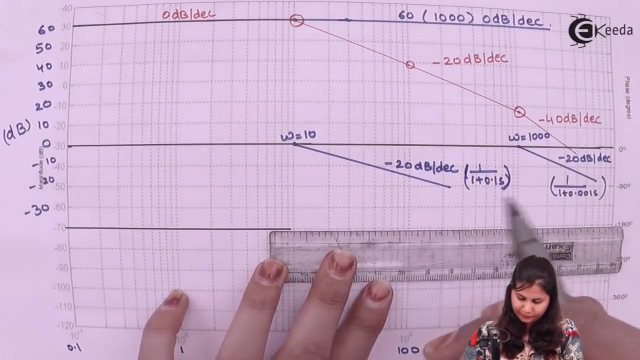 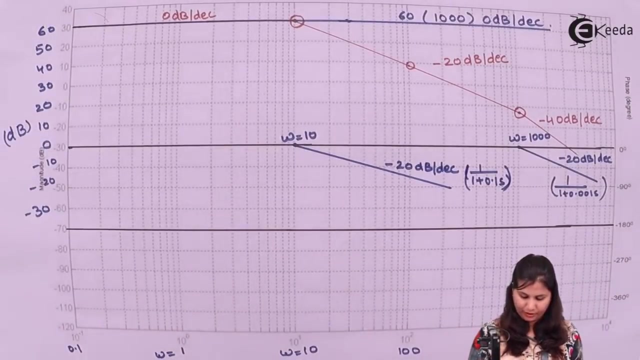 we will draw the line minus 180 degrees, okay, and phase angle: we are going to draw- okay, this is minus 180 degrees- line. make it as the reference line. now. for omega equals to: we will use the phase table. for omega equals to 0, the phase angle. 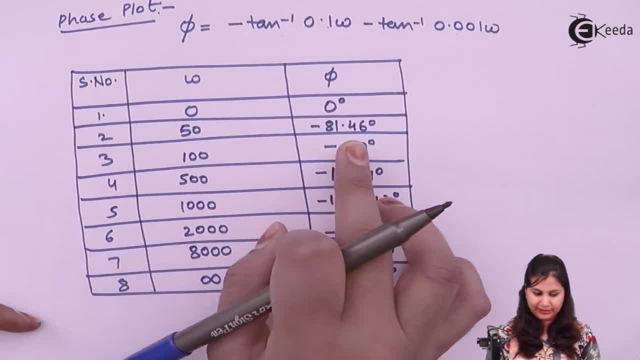 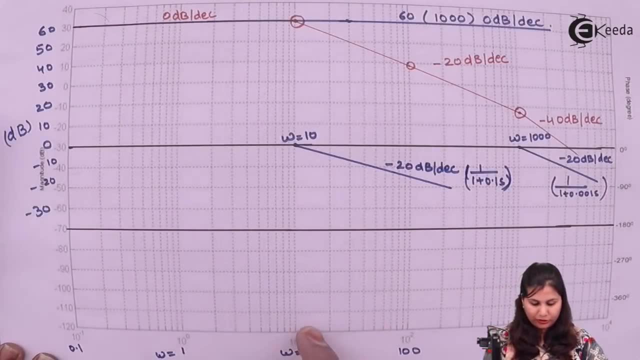 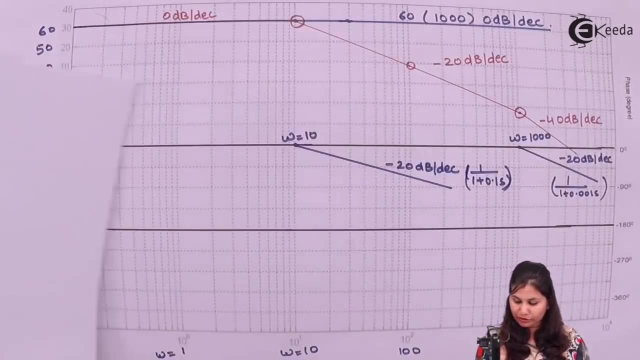 is 0 degrees for omega equals to 50. the phase angle is minus 81.46. so let's choose the table, because here we are having the frequencies we have chosen, up till 2000- 8000. so we are for this phase plot, we are going. 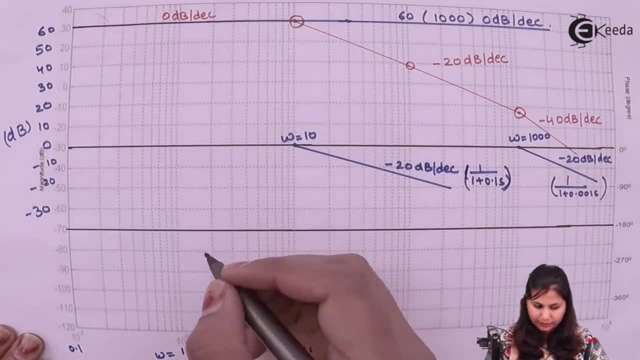 to change the frequency scale. mark this as this is 10, so this will be 10 here. first step will be plus infinity and then as far as the value of slots, these are total rupees, and then we appointed as honest to do it like it is now okay, as always. the line here: 80 degrees. this is minus 70 degrees. so change the frequency scale and we are going to use the frequency values, line 10. so that means we are going to change up to 10. other side, as if you are gonna see divided the scale of the yeah and 80 degrees is mostly undefined. so here the right side 1. 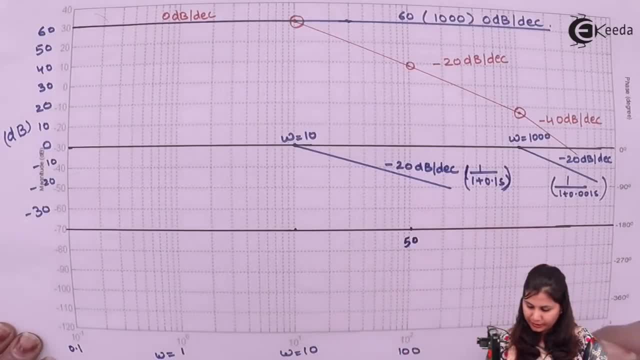 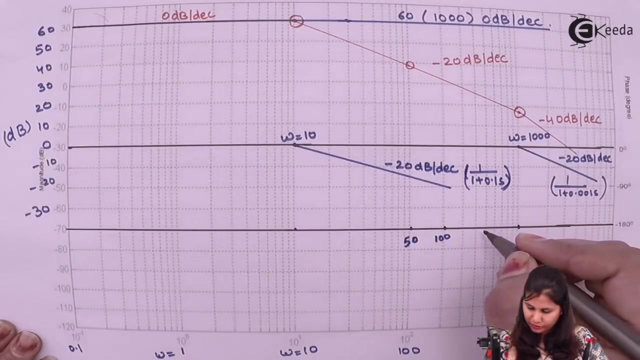 as 10 z feels like modulating the line. but here you can drunk, so we are going to toppings, an 50, then this will be 100. here we are going to have 10 raised to the power 3. so this is 10 raised to the power 3. so here we are going to have 500, then this will be 2000, then we 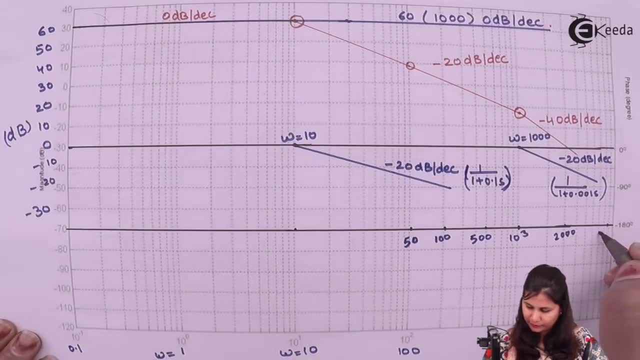 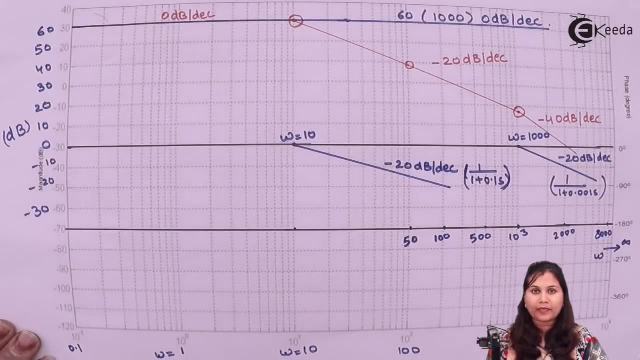 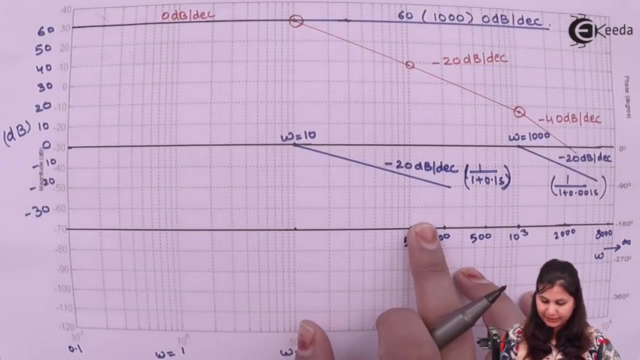 are going to have 8000, let us suppose here is 8000, and then we are going to have infinity Omega. so choose the scale, mark the points. all so for omega equals 250. the phase angle is minus eighty one point four, six. so minus ninety is here, minus 81 will be somewhat here. 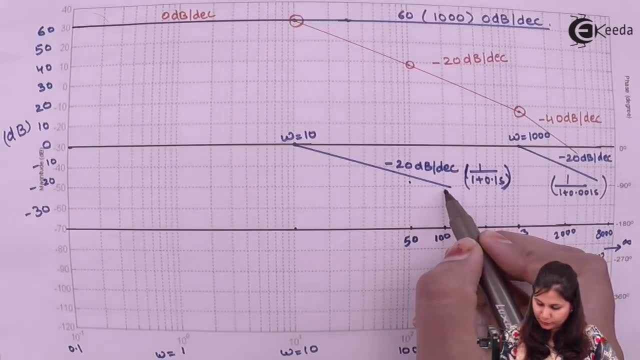 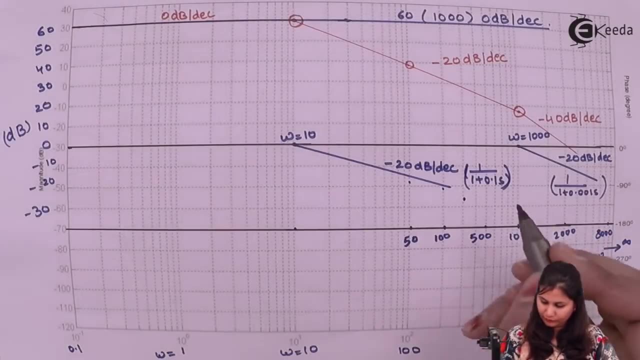 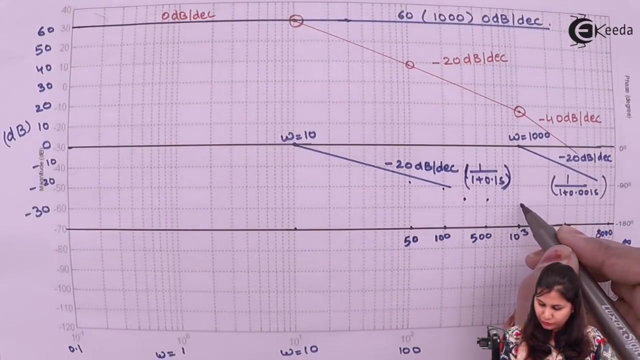 for omega equals to hundred, the phase angle is 90 degrees, so it will be here. for Omega equals to 500, it is 115.. 115 here For omega equals to 1000, it is minus 134.. So 134 will. 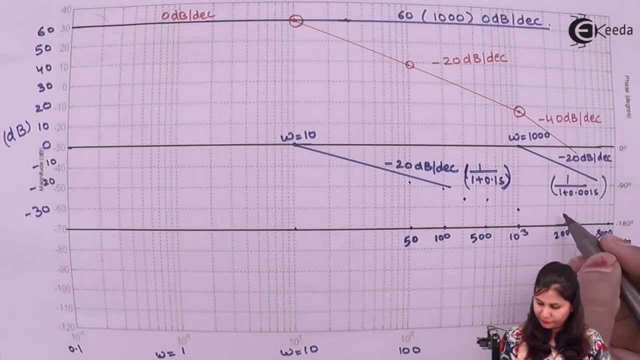 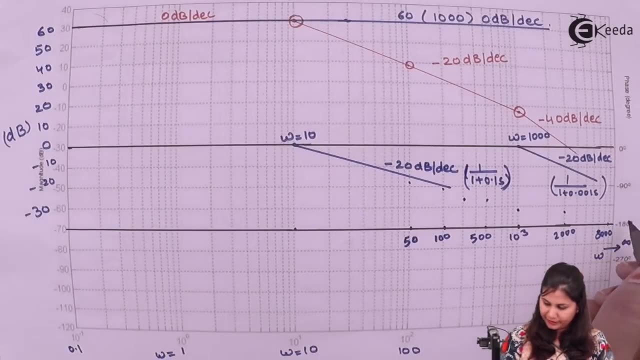 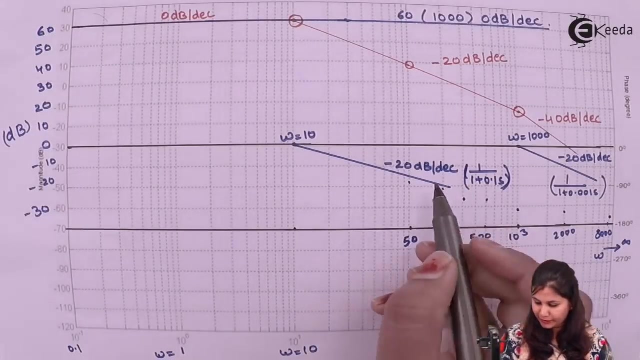 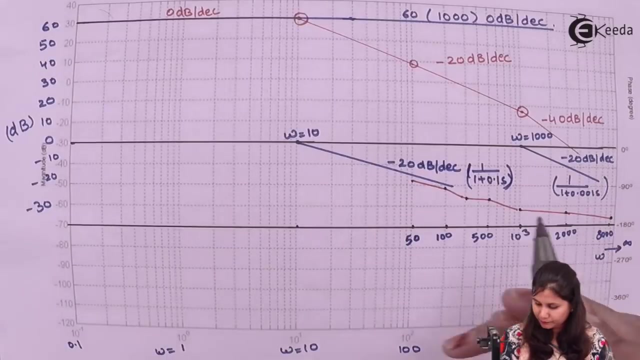 be here. For omega equals to 2000,. minus 153 degrees. Choose a proper scale for this. For omega equals to 800, we have minus 172.. So we have all the points. Just join it so that we will get the complete phase plot. Now, when this magnitude plot, because we have 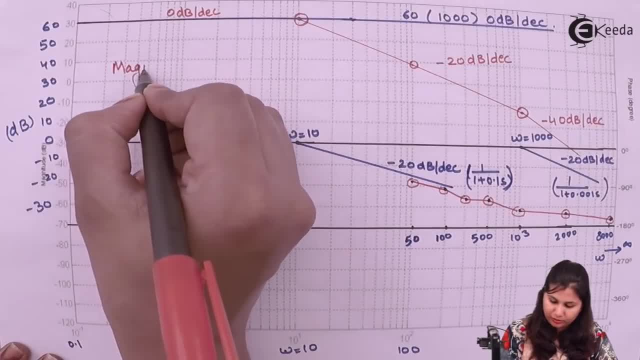 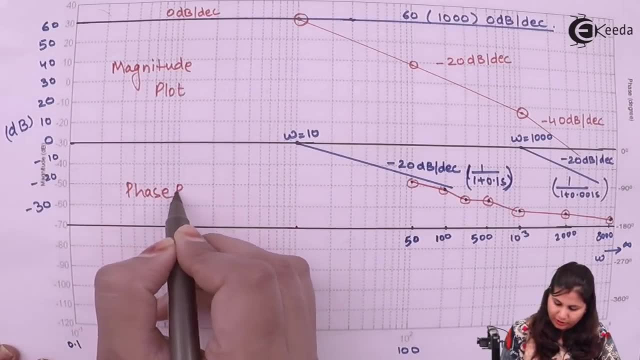 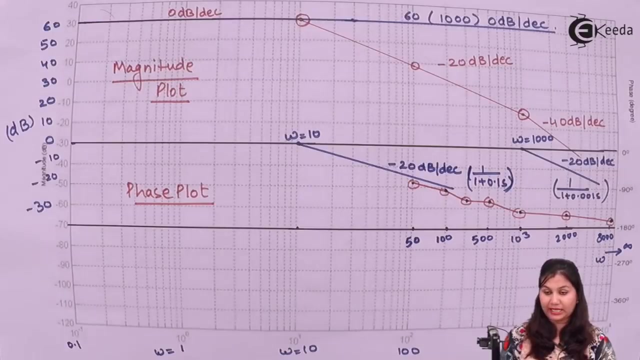 to calculate. this was our magnitude plot and this is our phase plot. So this is our phase plot. We have sketched the complete board plot. Now to calculate the phase margin: gain margin, phase crossover frequency and gain crossover frequency. we will check that. 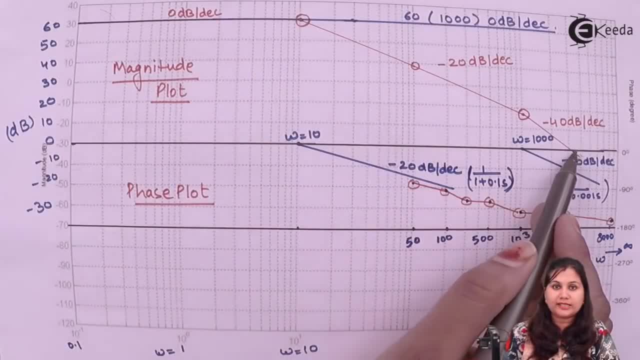 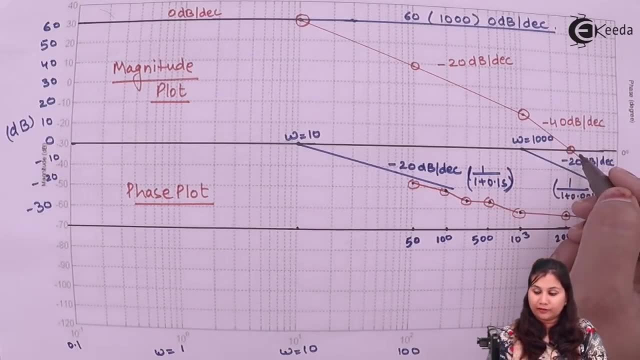 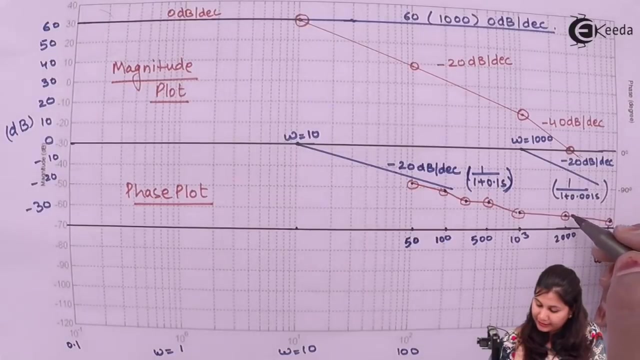 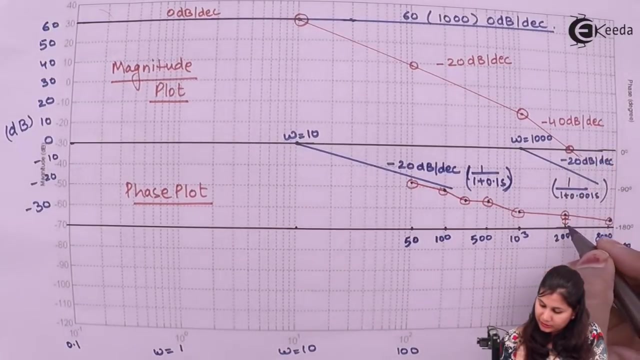 where this magnitude plot is intersecting with the 0 dB line. So this is intersecting at this frequency. So this frequency will be the phase crossover frequency and the angle at At this. this will be phase crossover frequency and when it is touching the 180 degree angle. 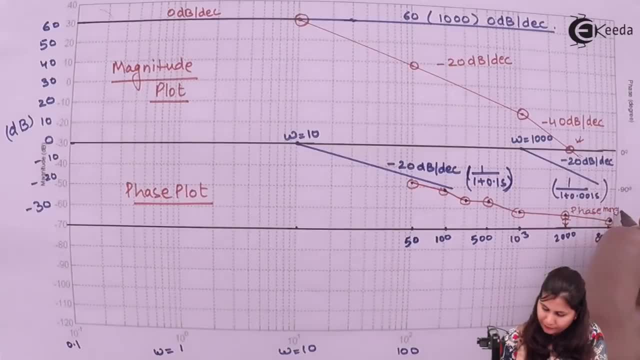 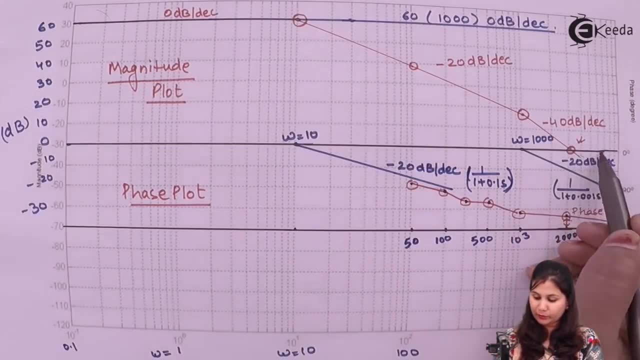 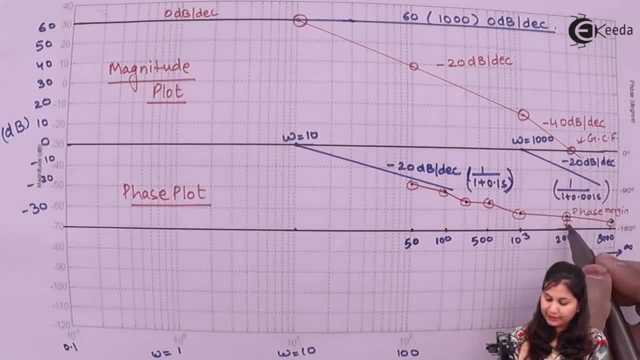 So this is the gain margin. The gain margin is called the gain crossover frequency and the phase angle at this is called the phase margin. So this phase margin will come out to be plus 21 degrees. Now for calculating the gain margin. we will have to see that where. 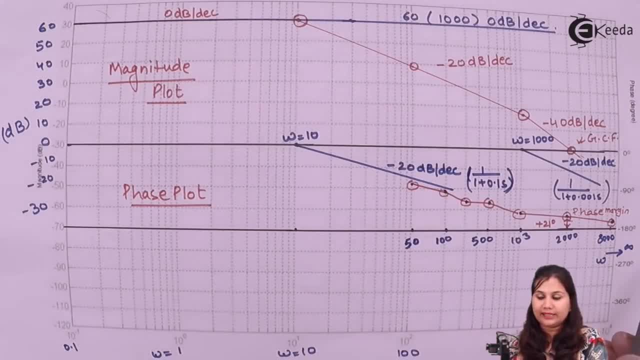 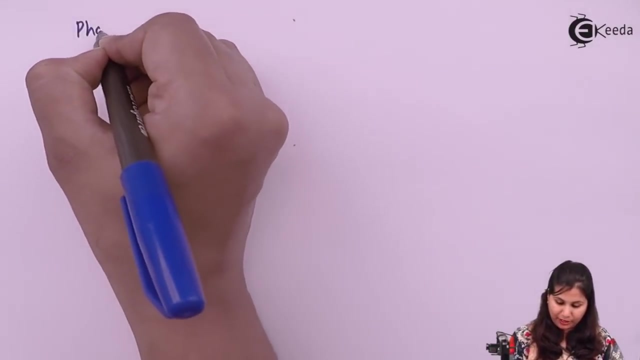 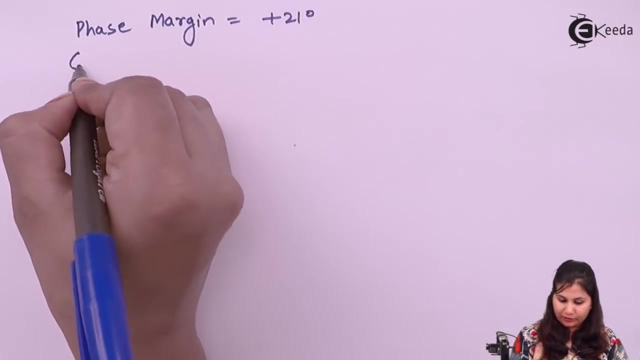 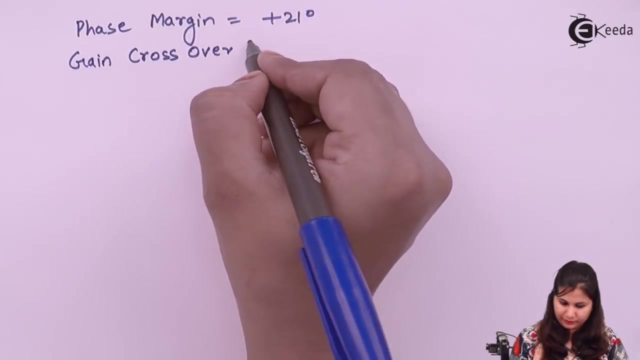 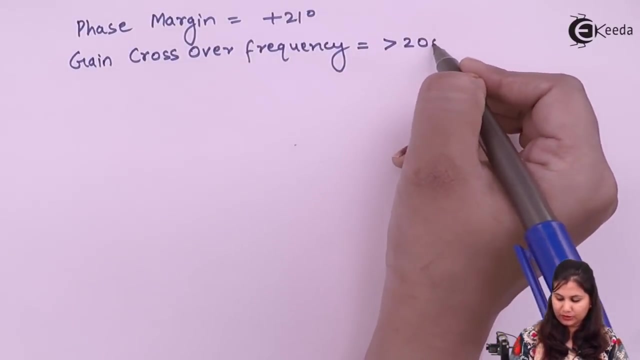 this phase plot is touching the minus 180 degrees line. So here it is touching this minus 180 degree line at infinity. So gain margin will be infinity here. So let us check, Check that. what are the values? We have phase margin as plus 21 degrees Gain crossover frequency. It will be somewhat greater than 2000.. Okay, And gain margin is infinity. 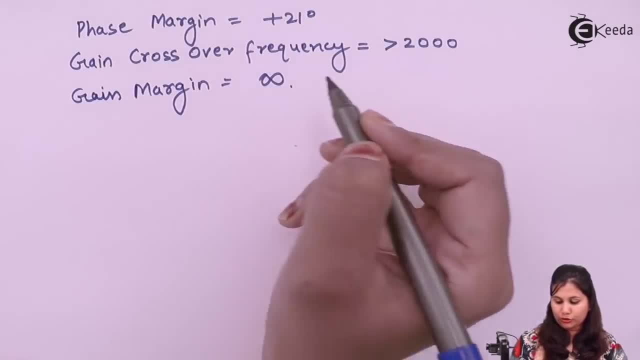 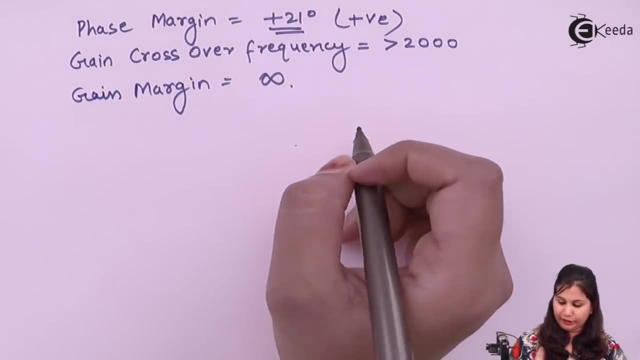 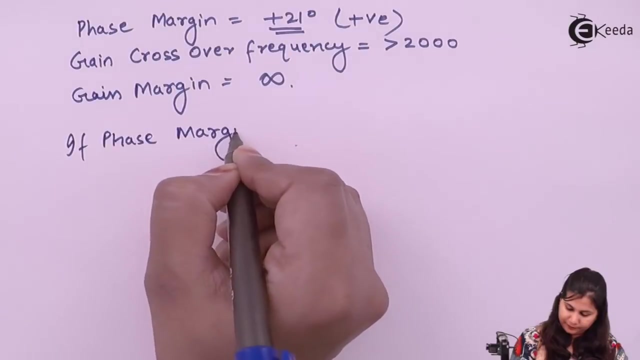 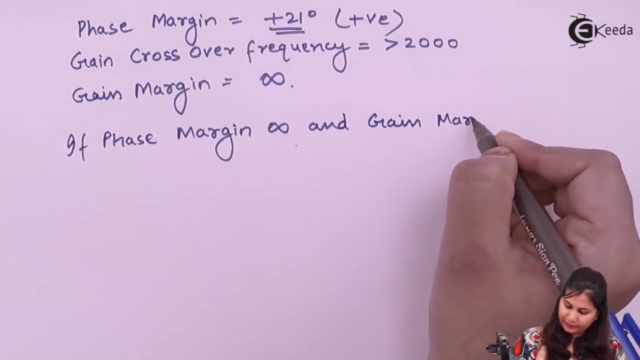 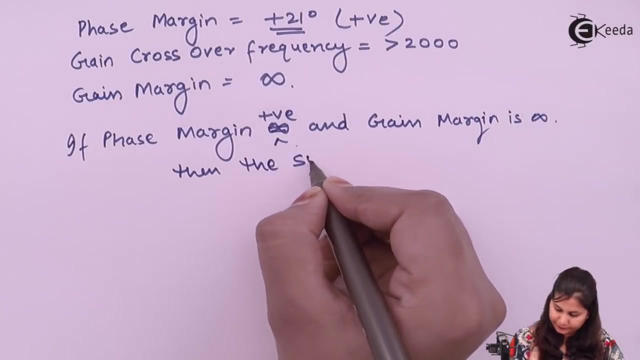 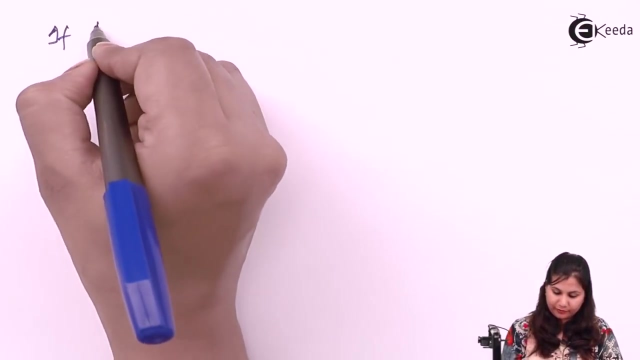 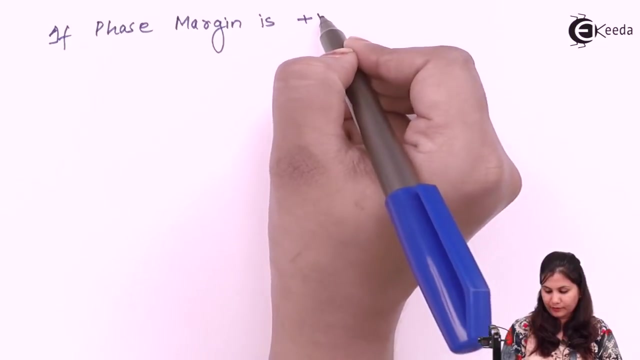 Okay. So you can see that this phase margin is coming out to be positive and gain margin is coming out to be infinity. So if phase margin is positive and gain margin is infinite- Sorry, phase margin is positive, Gain margin is positive, Gain margin is infinity- Then the system is inherently stable. So if phase margin is positive and gain margin is infinity, 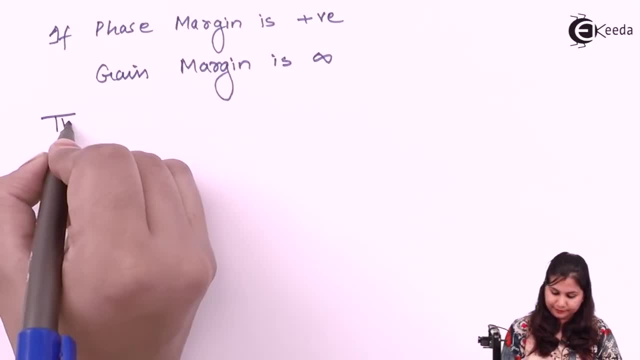 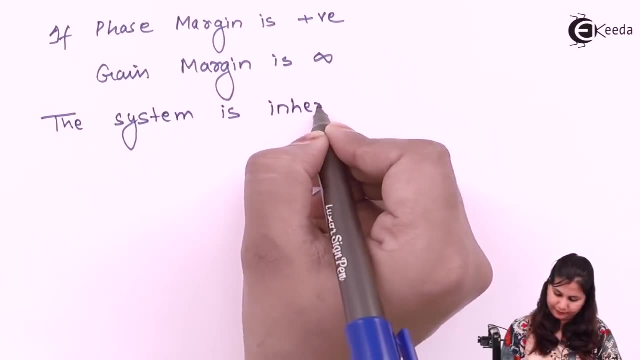 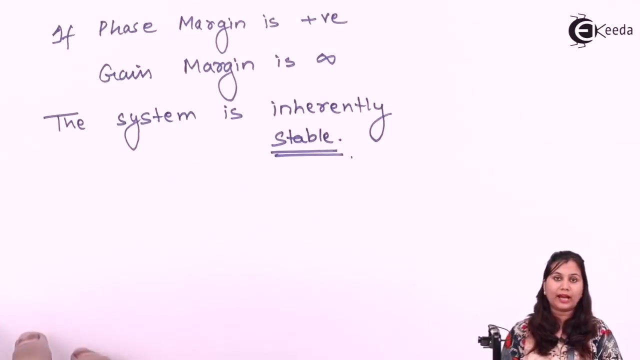 The system is inherently stable. So in this problem we have sketched the boat plot of the system and we have calculated the gain margin and phase margin and also the stability of the system. So what you have to do whenever you see the, the questions on the board plot, first put s equals to j, omega, so that you can be able to.